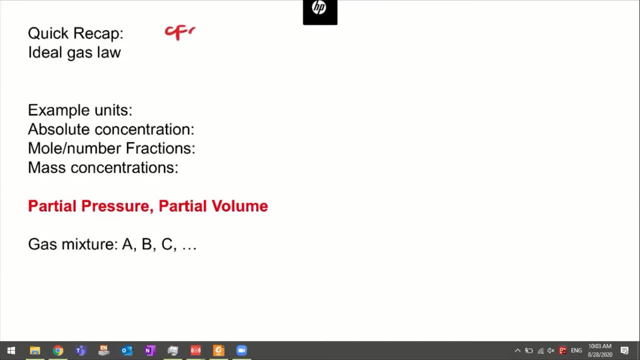 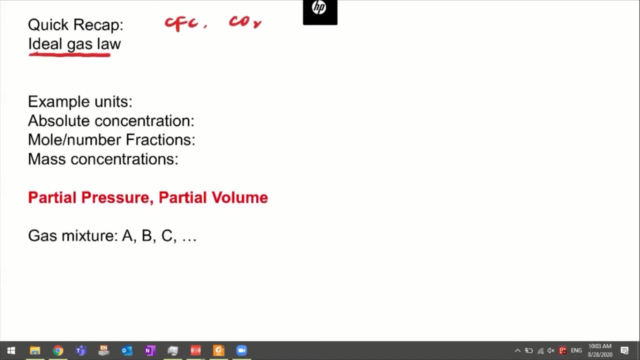 chlorofluorocarbon, the CFC right, and also we mentioned a little bit about carbon dioxide, which is causing the global climate change, And then we mainly talked about the ideal gas law. So we use that to convert different units, right. 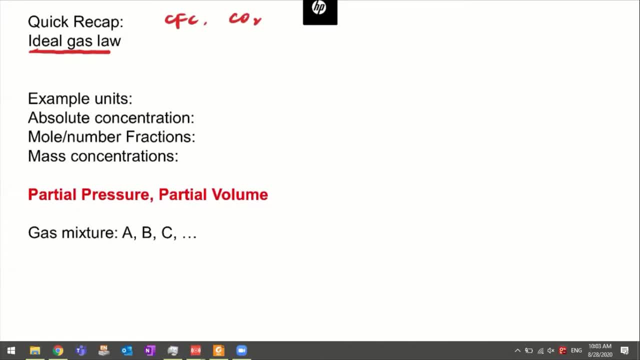 and so the example units can be absolute concentration, mole or number, fraction and mass concentrations. So we mentioned about the partial ideal gas law, which is basically NA divided by NA, RT equal to PAV, right, so let me just quickly Alright, so okay, so basically we can use this ideal gas law to calculate the to. 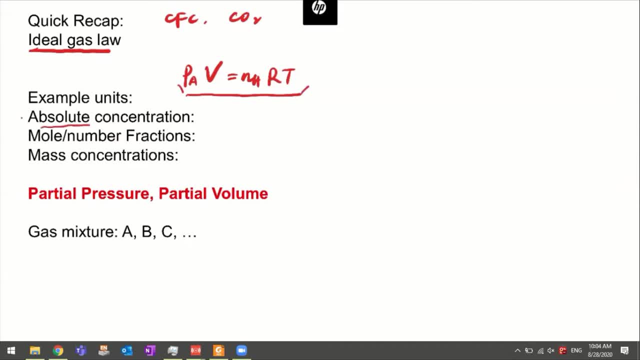 basically convert all of these units. right? So we know that the absolute concentration can be represented by NA divided by V. That mainly that's the issuits for the scenario when we're trying to calculate like, say, mole per liter or mole per meter cubed, so on and so forth. right? So in terms of the 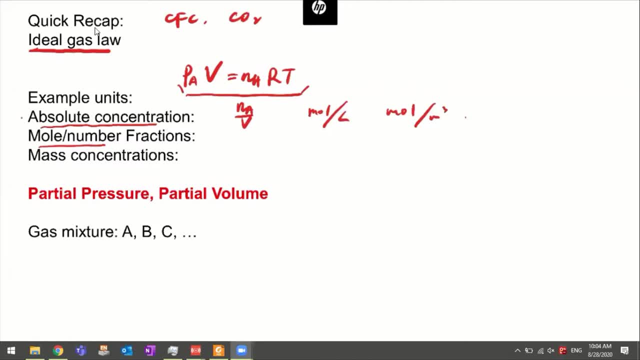 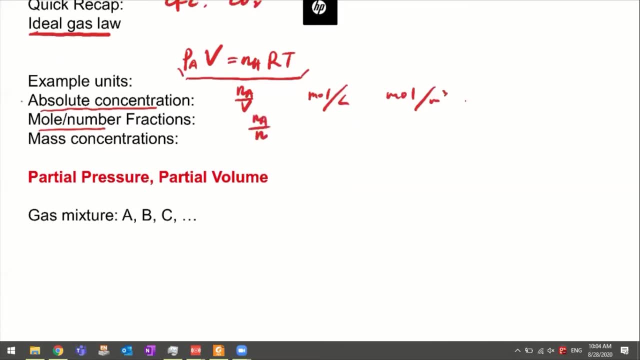 mole or number fraction. that's going to bethat's going to be NA divided by N, right, So the mass concentrations will be MA divided by V. So these are the different types of units to represent the concentrations of gas, species or air. 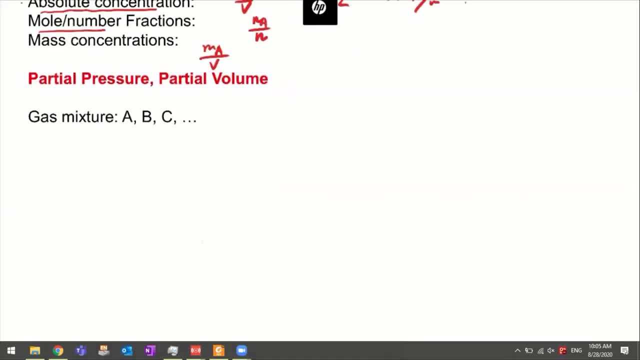 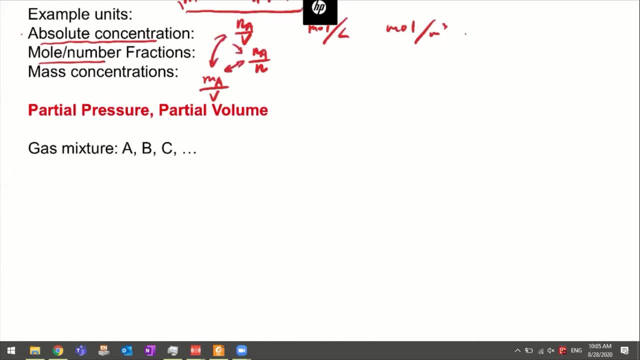 pollutants. I will also introduce how we can convert different units right? So basically we're trying to convert from one another in here. So actually it's quite easy to directly convert the absolute concentration into mass concentration, mainly because Na can be calculated by Ma divided by the. 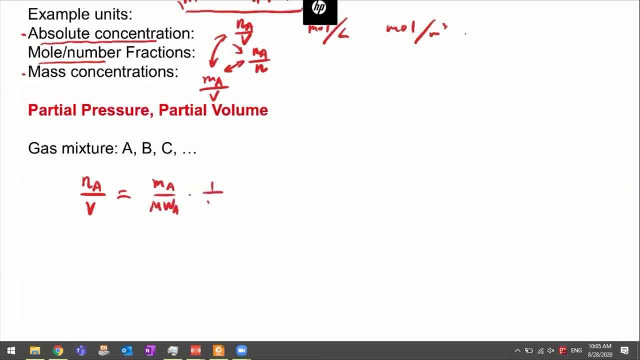 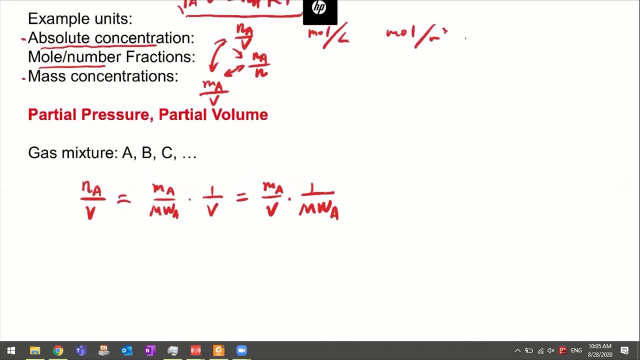 molecular weight of A multiplied by 1 over V. right, So we can write that. write that out as Ma divided by V multiplied by 1 divided by molecular weight of A. okay, So the thing is how we can convert from or between these two. So if we write: 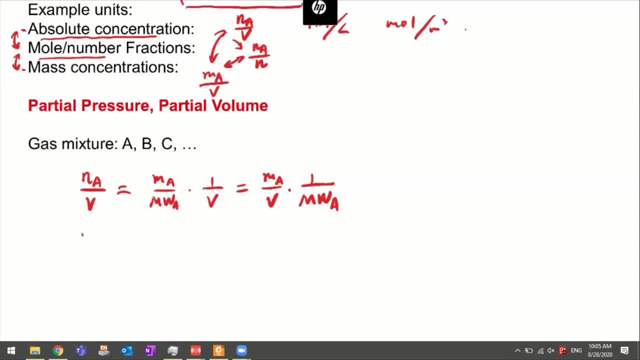 out the, let's say write out this absolute concentration again. So we know that ideal gas law works as PV equal to nRT, right. So we can have V equal to nRT divided by P. So we can plug in this volume term into here and you: 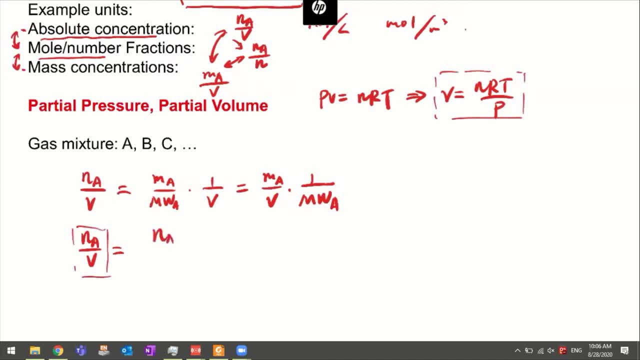 can find out that this actually works as Na divided by N, multiplied by RT divided by P. okay, So now we converted this absolute concentration into mass concentration. So we can write that, write out this absolute concentration into the mole fraction. okay, And since we know the relationship, 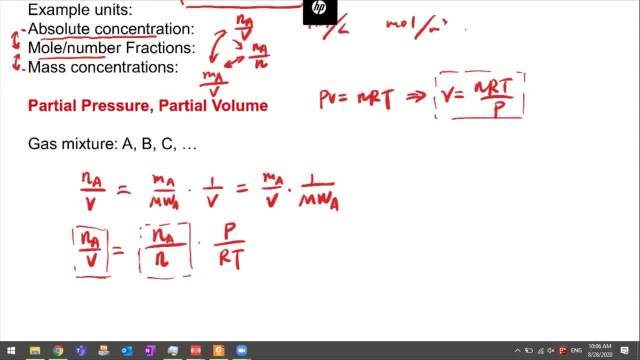 between. so basically, we know the relationship between the mass concentration and the absolute concentration. we can also further do a step to convert this into the mass concentration, right? So that is done by? if we write it out as: Na divided by N, multiplied by P. 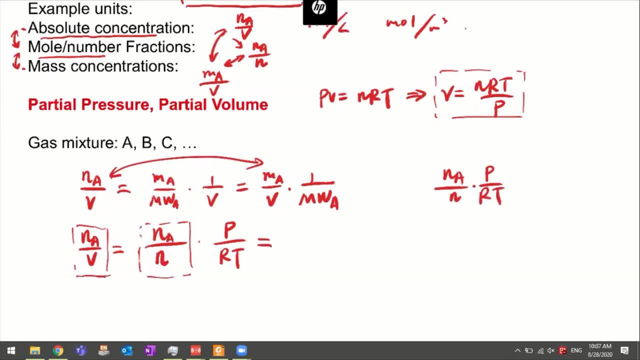 divided by RT, which is equal to this term, And that's further equal to Ma divided by V multiplied by 1, over molecular weight of A. So we know that basically, the Na Na divided by N is going to be equal to Ma divided by V multiplied by RT divided by P multiplied by V. 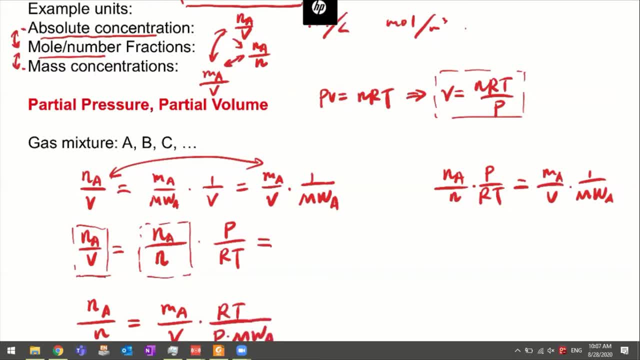 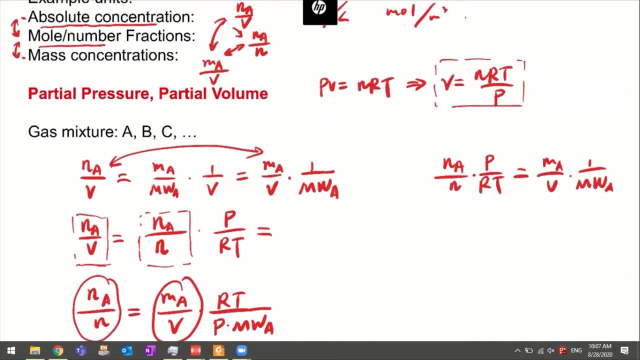 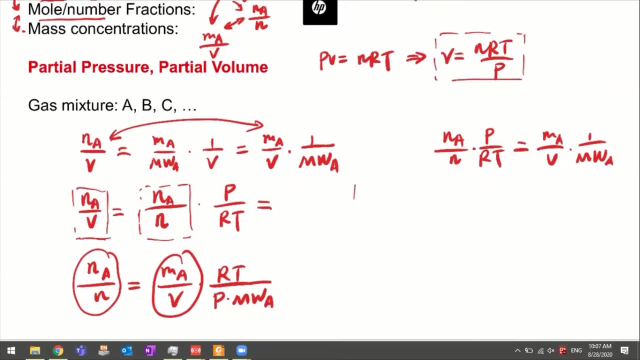 molecular weight of A. okay, so this is how we can convert from the mole fraction into the mass concentration. all right, so let's say, if we write on all of these equations- although I think it's a little bit boring to go through all of these derivations, but it's going to be quite useful- or straightforward when. 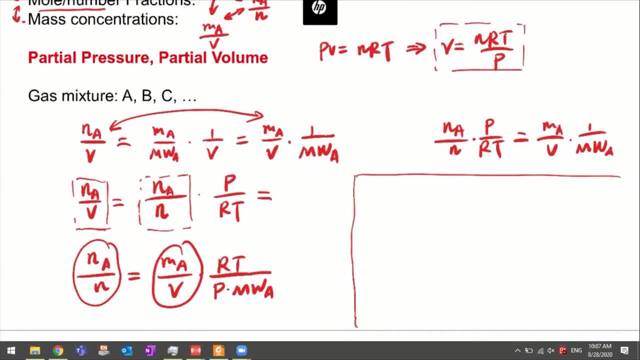 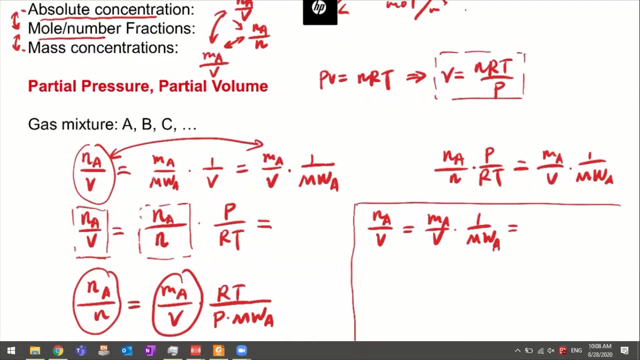 we're trying to convert different units, okay, so let's start from the absolute concentration. we know NA divided by V is equal to MA divided by V multiplied by 1 over molecular weight of A right. so how do we convert this into a mole fraction? so basically we also have here, have it here, right. NA divided by V is equal to: 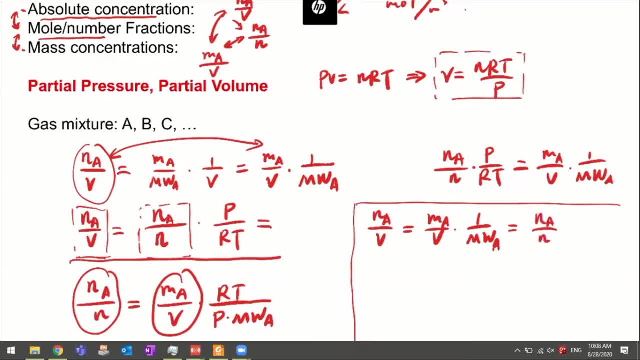 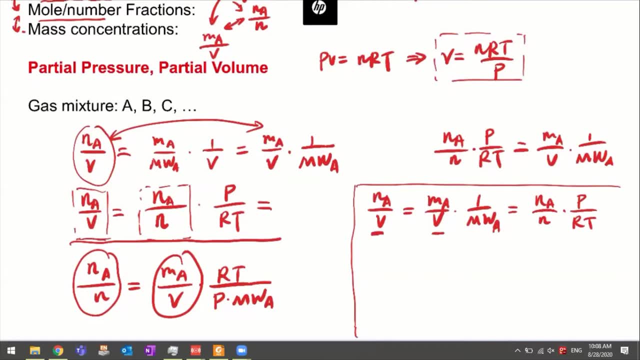 this term. so NA divided by N multiplied by P over RT. okay, so this is absolute concentration, this is mass concentration, this is mole fraction. okay, and similarly we can write it out as: MA divided by V is going to be equal to NA divided by V multiplied by molecular weight of A, and this is also 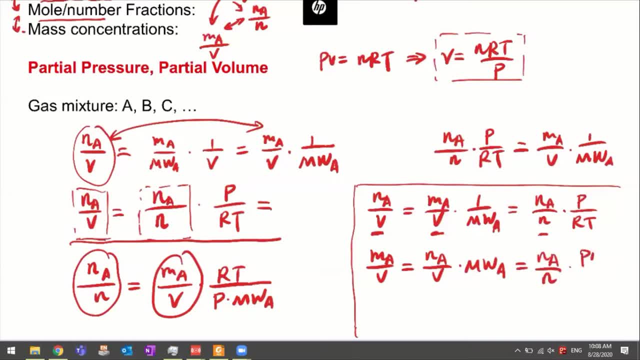 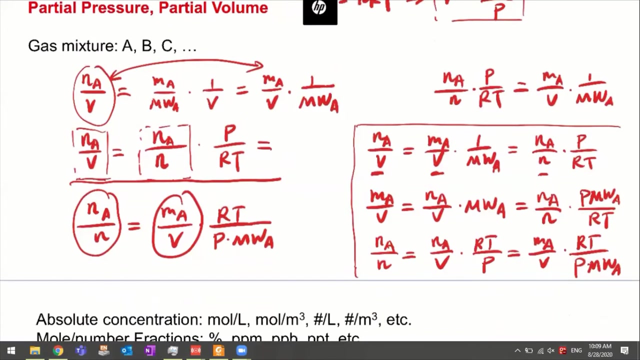 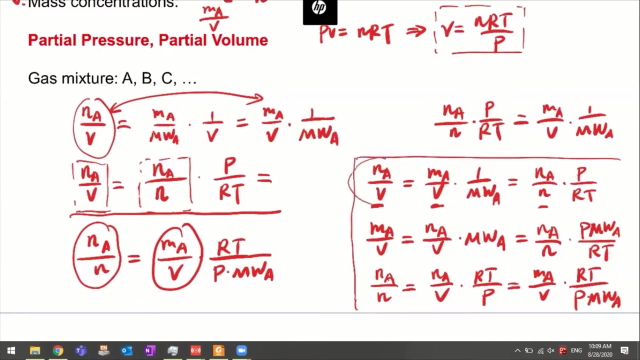 equal to NA divided by NP, multiplied by molecular weight of A divided by RT. finally, we have a: M is equal to N, A divided by N equal to NA divided by N. okay, it seems a lot of equations here, but the main one, basically, if we know how to convert from one another, from one set of equation, 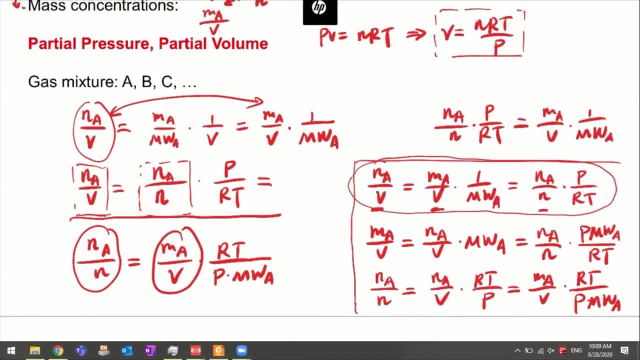 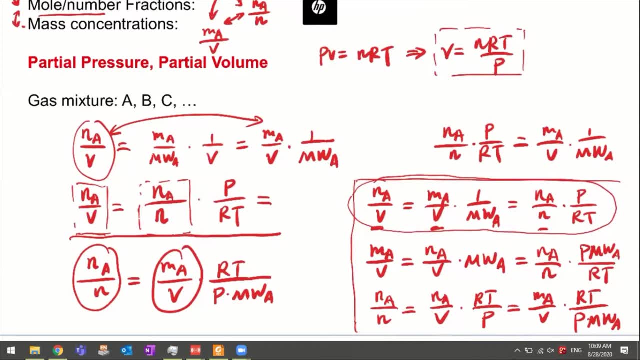 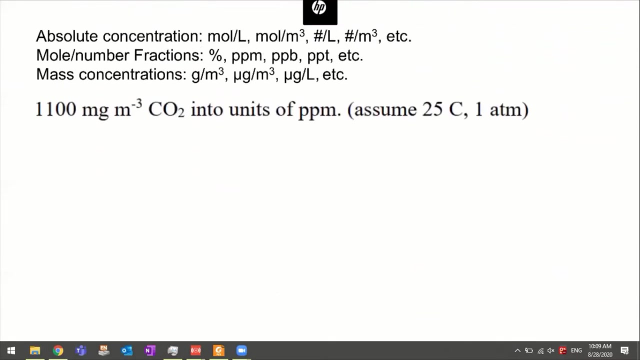 we should be able to derive the rest of them, right? So I'll wait for everyone to finish. Good, So let's try to apply this, all right? So here's an example. So let's try to convert 1100 milligram. 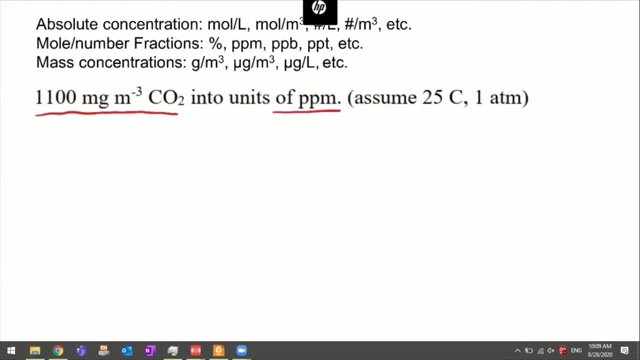 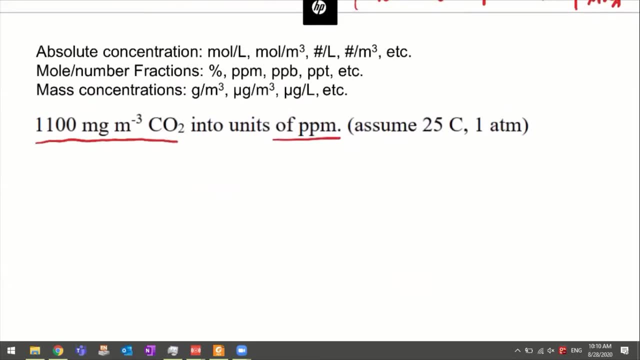 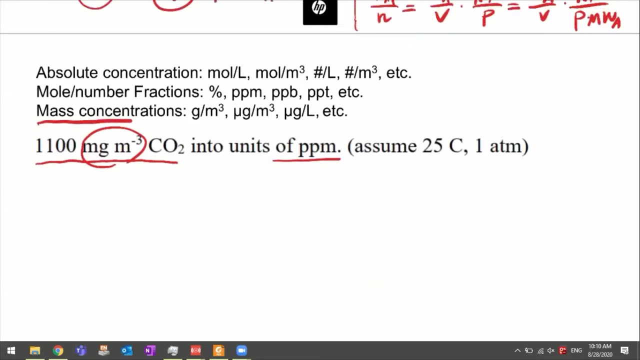 per meter cube of carbon dioxide into the units of PPM. So what does that mean? So, basically, we know a concentration of the gas species with a unit of milligram per meter cube And we know that by having a unit like this, it's gonna be the mass concentration, right? 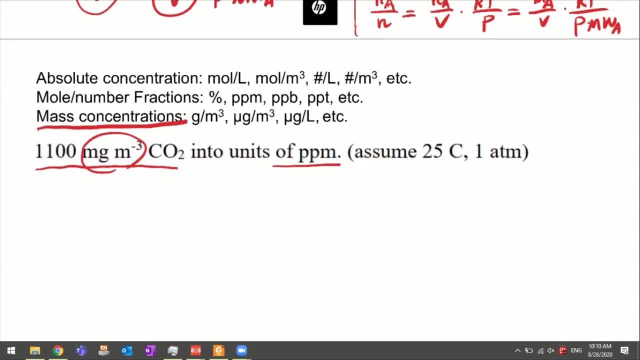 So we're trying to convert from mass concentration into mole or number fraction. So basically, what we're trying to do is MAD divided by V into NA divided by N. okay, So we don't know what this term is, So which equation we should use. if we look at this, 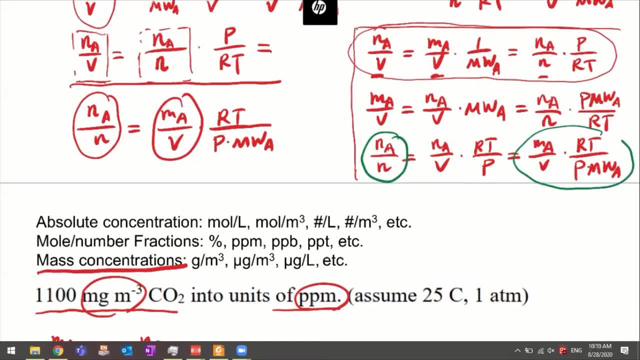 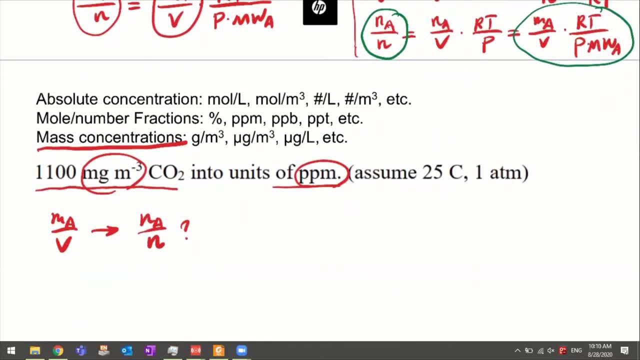 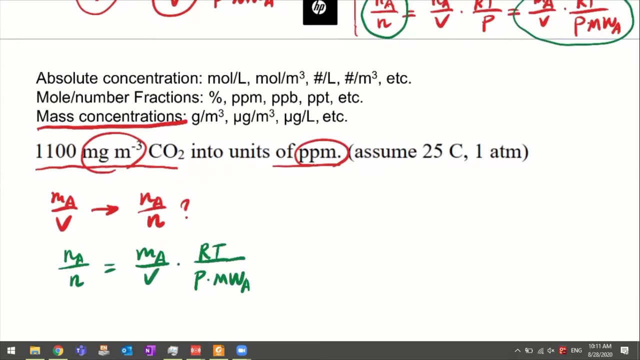 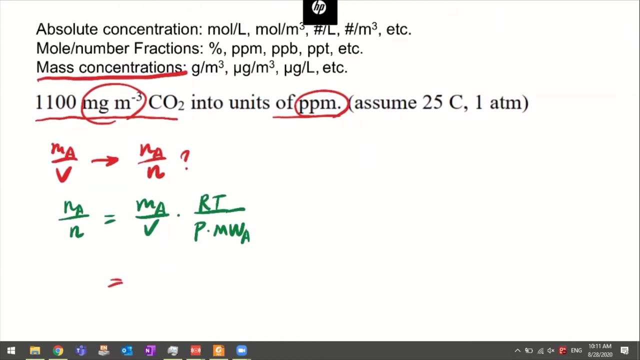 So we should use this one right. So we should have NA, divided by N, equal to MA, divided by V, Multiplied by RT, divided by P, molecular weight of A. okay, So now we can try to plug in all of these numbers, because we know that the mass concentration 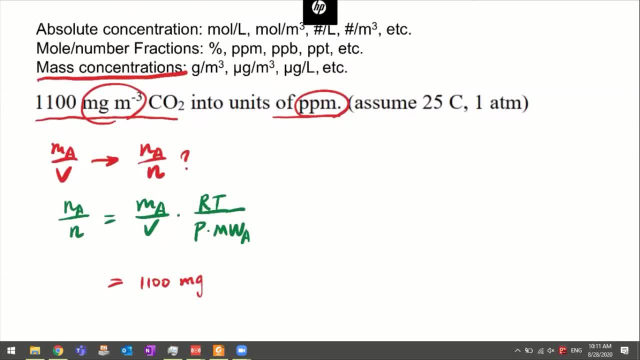 is 1100 milligram per meter cube, right, And then the R is equal to 8.314 joules per meter cube. Okay, So we can use that to calculate the mass concentration if we want to convert it into Kelvin. So if we look at the temperature, 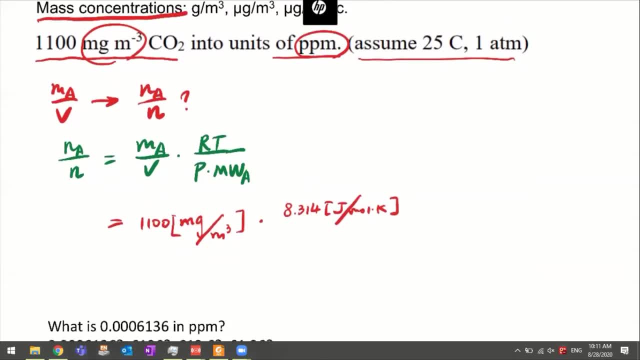 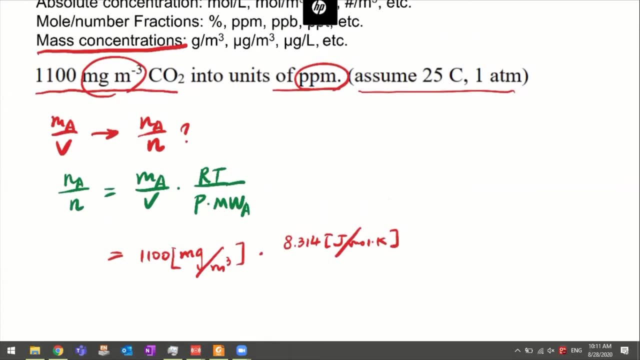 the temperature. in the ideal gas that's gonna be 1.926 joules per mole per K. So here we also assume certain temperature and pressure. All right, So if we have 25 Celsius we need to convert that into Kelvin, because in terms of the temperature, 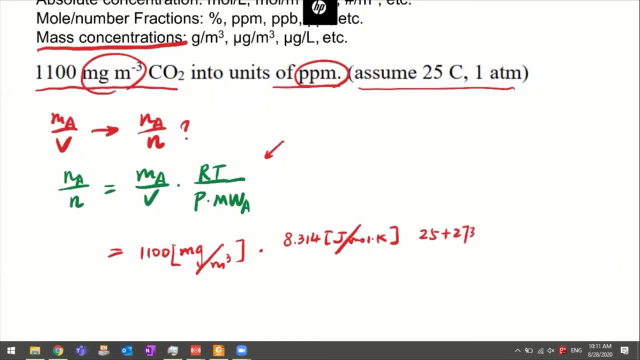 in terms of temperature. in the ideal gas law we have to use the standard units, right? So 25 Celsius is gonna be 25, plus 273.15, and divide by. for pressure we have to use the Pascal 1.01 multiplied by 10 to. 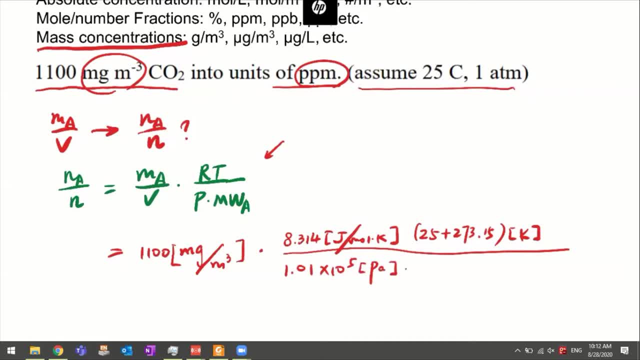 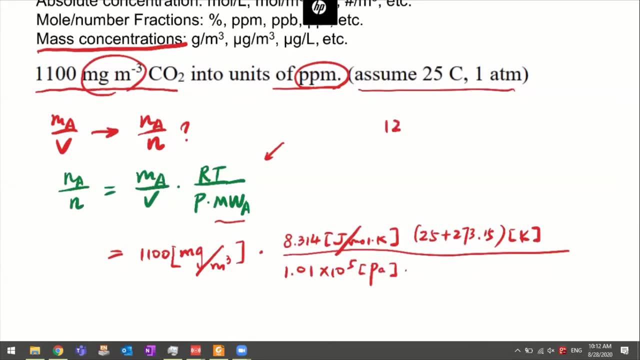 the fifth Pascal. and then we need to know what is the molecular weight of carbon dioxide. So we know carbon has a molecular weight of 12,. oxygen has a molecular weight of 16, we need to multiply that by 2 to get 44.. 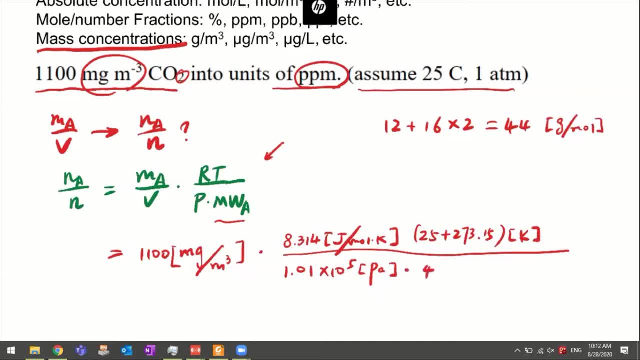 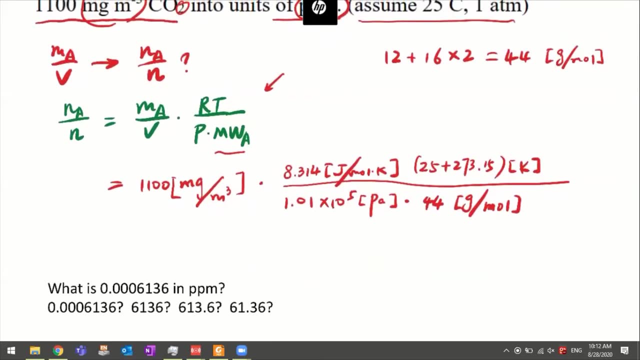 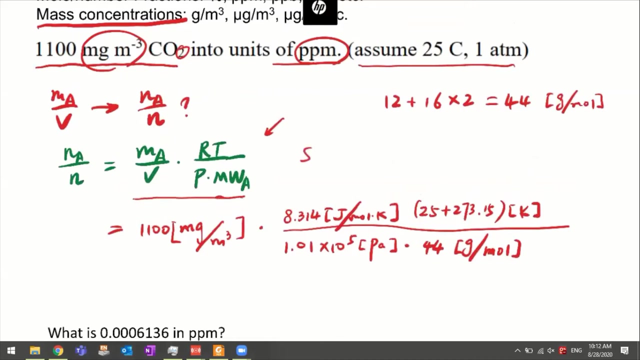 So we multiply 44 gram per mole. Alright. so now what we need to do is check the units, because we cannot multiply everything together. Because we know that for ideal gas law they have to use the standard units. so we know that for the mass, constructors. it needs to be below the base beta and negative sigma, and so we need them tocal in water balance So we can justify thevector of the到底 togain the rate of dispute. uh, as a carbons gem of a, кстати認為 i. so we nowora deriva United Way, we can use the reframed formula for the gas structure, since we don't have a standard unit. So what is invert? 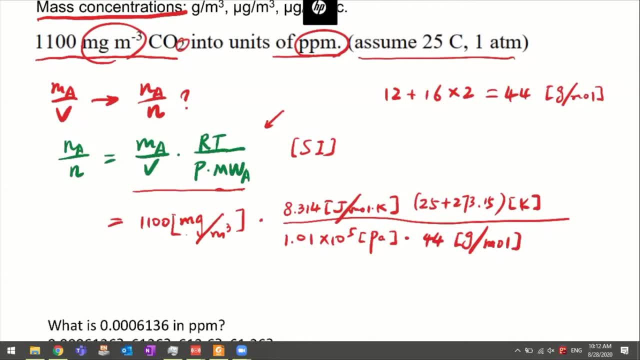 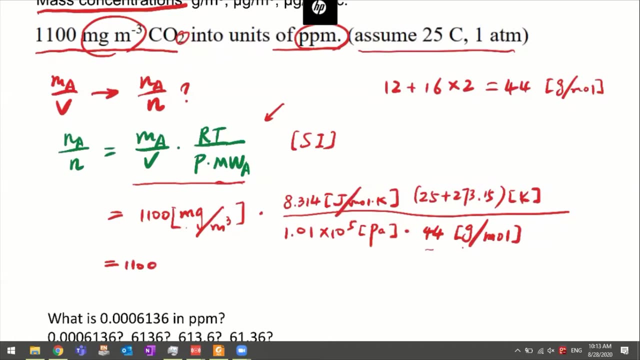 Concentration. here We're talking about the milligrams and also here for the, for the molecular weight, We're using grams. We need to first convert all of them into standard units, so We'll keep the 1100 number here. but we know that one milligram is equal to 10 to negative 3. 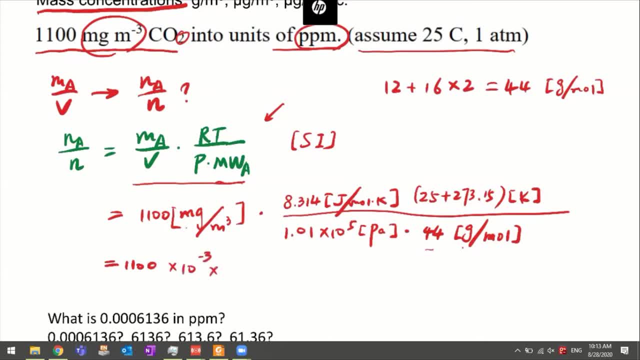 grams and To convert that into kilogram We need to further multiply by 10 to the negative 3. In this way we have kilogram per meter cubed. Okay, and similarly at here, eight point three, one, four, true, will promote Okay, Multiplied by two, ninety eight point one five, Kelvin. 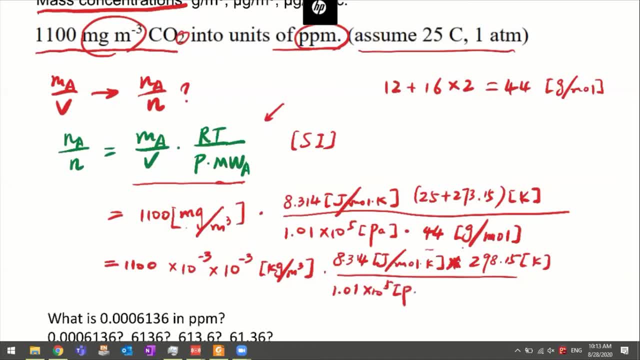 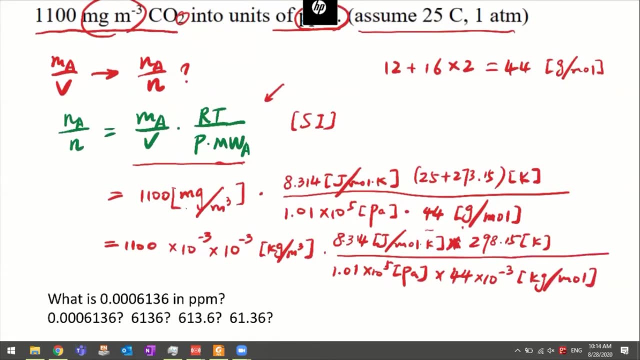 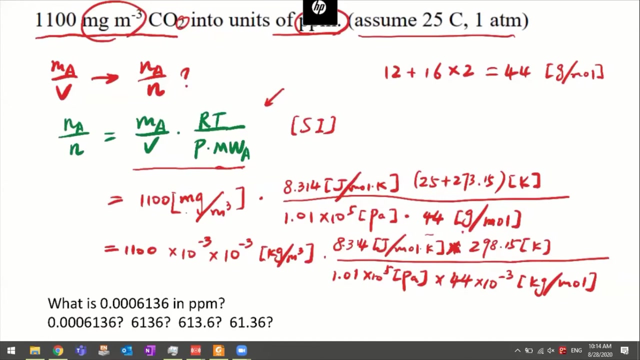 One point, oh one, multiplied by 10 to the fifth Pascal. So We also converted this gram into kilogram here. all right, so in this way all of the units should be able to conserve. and Let's also check the units. Okay, so we know that here are a lot of units showing up and 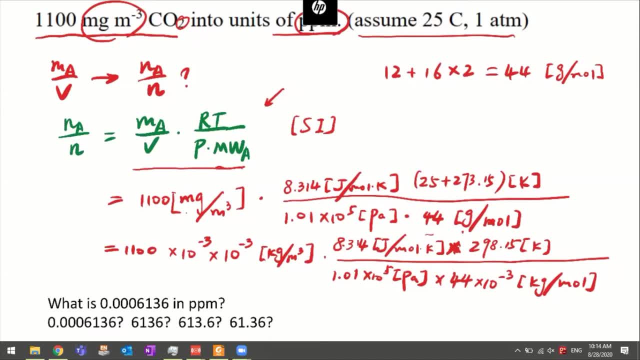 We need to cancel them All right. so we have Kelvin and Kelvin get cancelled right, Mo per mole and per mole getting cancelled right, Kilogram and kilogram getting cancelled Right. So finally, in terms of the unit, They're going to have the unit of Joule divided by Pascal. 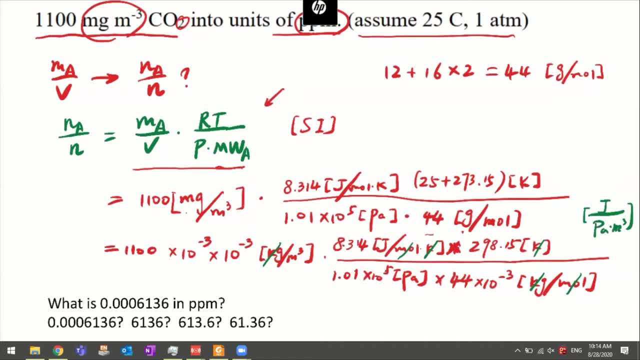 multiplied by meter cube. Okay, so this is. we're trying to summarize all of these remaining units here. So I think last time we showed that basically Pascal multiplied by meter cube has a unit of Joule. This is mainly because Pascal, that's Newton, divided by meter square, right? 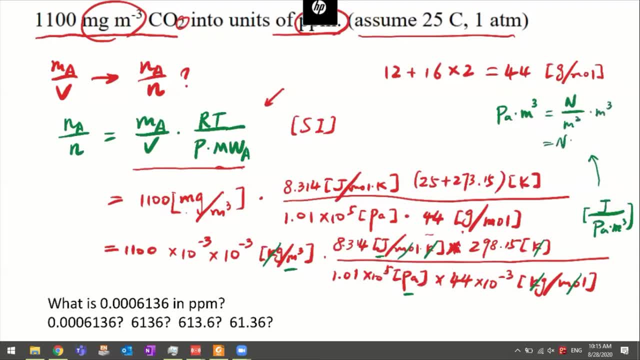 And if we multiply by meter cube, then that's going to be Newton multiplied by meter, which is Pascal, which is true. Okay, so everything should cancel in terms of the unit of Joule, And this is also the reason why we were getting more fractions, because fractions 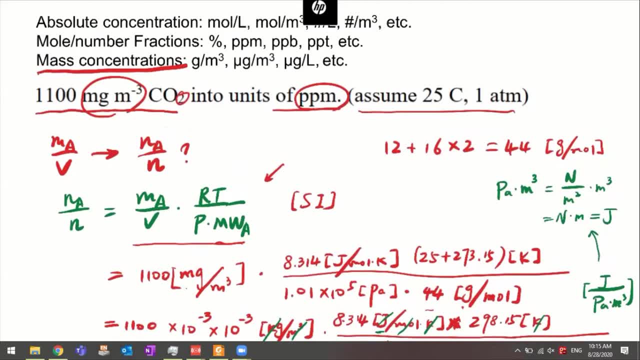 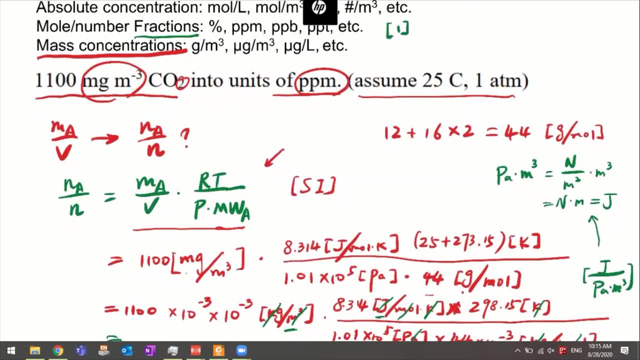 This is also the reason why we were getting more fractions, because fractions, They shouldn't have any unit, they should just have a unit of 1, because it's not number divided by number Shouldn't remain any units here. Okay, so now we can just multiply all of these number together. 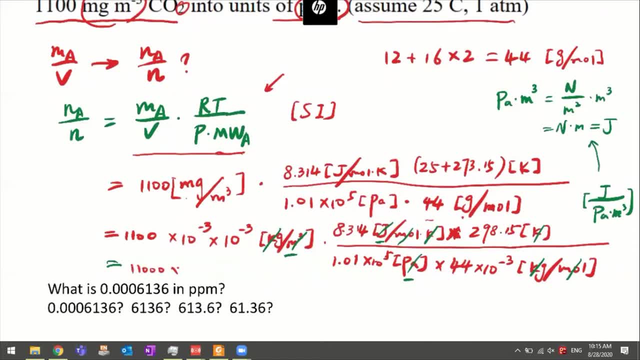 so it's 1: 1, 0, 0. Multiply by 10 to the negative. 6, multiply by 8.36, 0.314, 298.15, divide by 1.01,. multiply by 10 to the 5th. okay, So this is the. 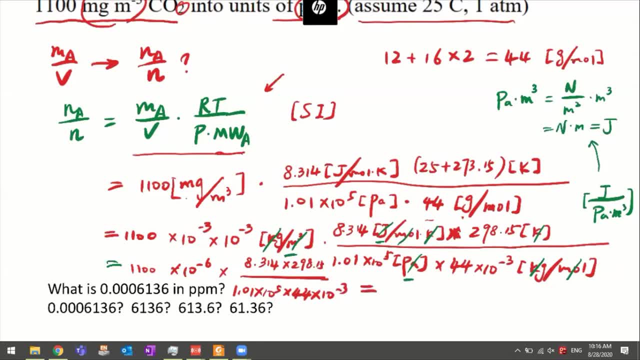 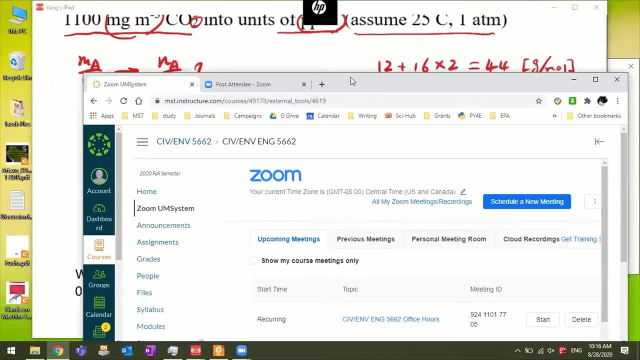 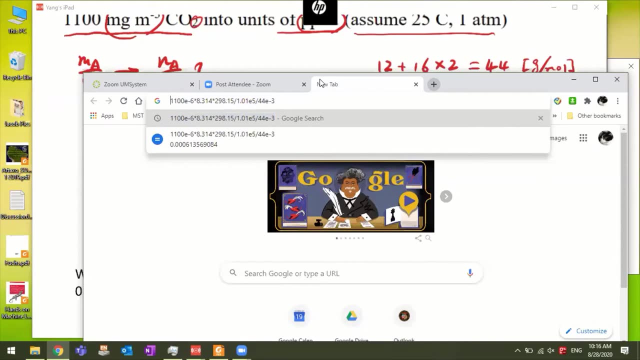 equation we're going to deal with. So if you have a calculator with you, you can start to type in, but here I'll just use the Google browser. okay, You have 1100, so I actually typed in this equation last night, So just trying to make sure. 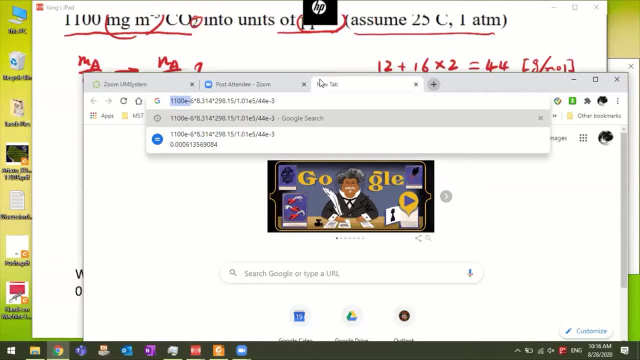 that we were using the right equation here. So 1100 multiplied by 10, to the length of 6,, 8.314, 298.15,, divide by the pressure and also divide by the molecular weight. So you guys can see this equation here right in the browser. 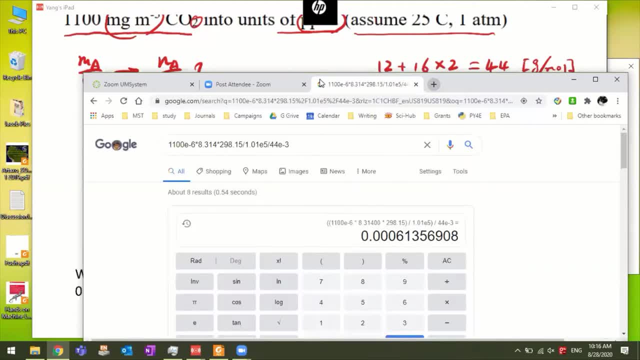 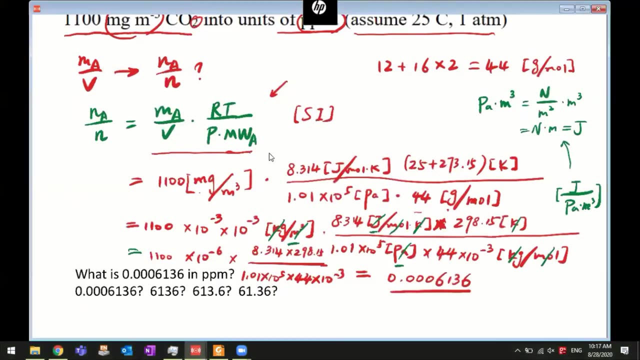 Yes, Okay, So this is what we get: 0.0006135,, 6136,. okay, So this is the mole fraction. And now, to make sure that you guys know what the what the PPM or PPT means, let's: 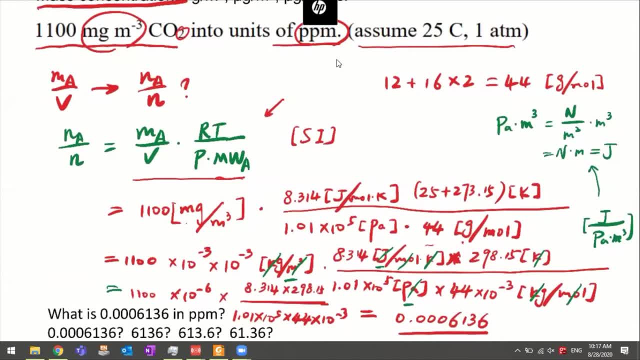 do a quick poll. So what is this 0.0006135?? So what is this 0.0006135?? So what is this 0.0006135?? And what do we get? This is 0.6136 and PPM, or parts per million. 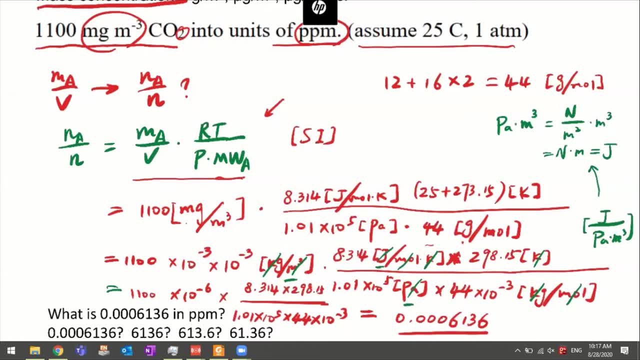 So we will give everyone percentage ofemetery and PPM. you can start to speak and then we will짚: y ns全 至. Okay, I'll just stop right here, All right. so still, most of you guys are correct. That's 613.6 ppm. 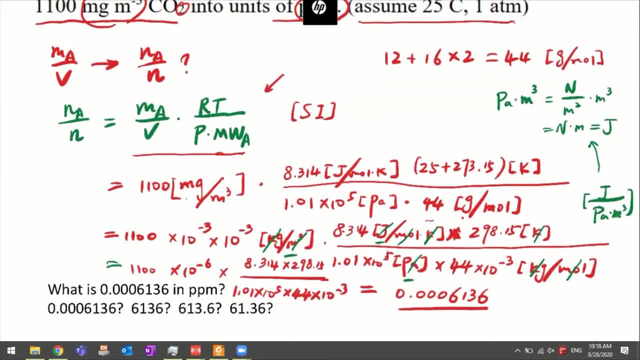 So when we say parts per million, we basically need to multiply this whole number by 10 to the 6th, Because 1 million is 10 to the 6th, right? So if you basically the digit should move up to here. 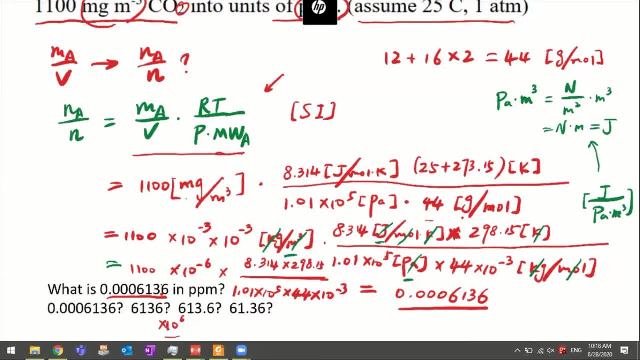 So it's going to be 613.6.. Right, We cannot directly use this number as in the ppm. So, similarly, let's say we're talking about the ppb. Basically, if we talk about ppb, then we need to multiply this number, this fraction here, by 10 to the 9th. 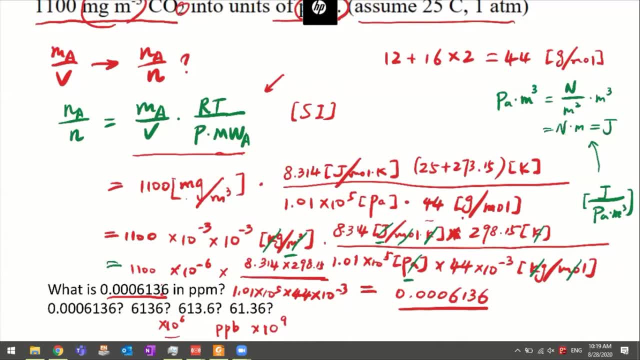 Right. So here we're talking about ppm, so we just need to multiply by 10 to the 6th, That's going to be 613.6.. All right, All right, Okay, so this is a quick example here. 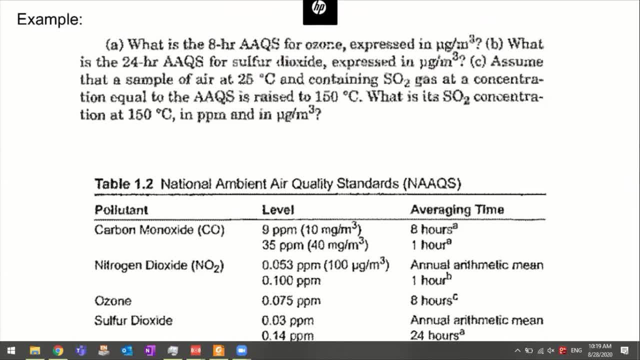 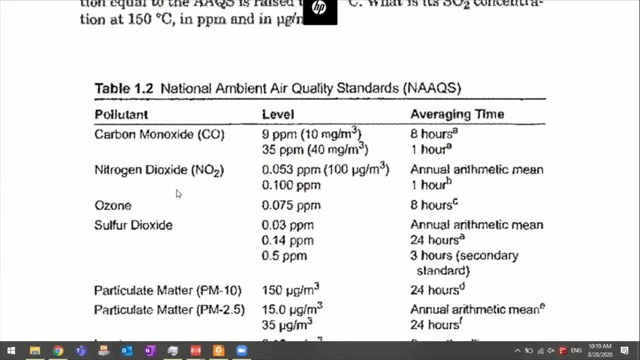 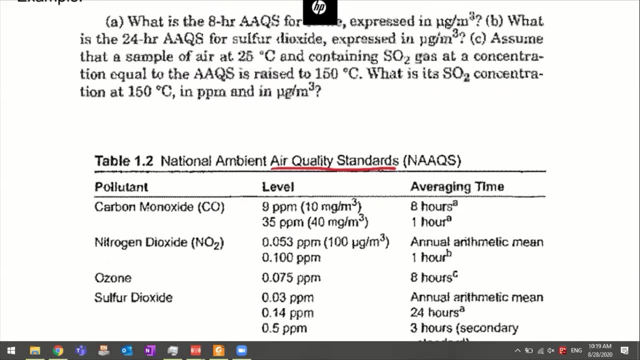 And now let's practice more. So let's get familiarized with this equation here, Right? So here I'm showing this table again. This is basically the air quality standard. different criteria, air pollutants- Right, And so this problem. let's first try to convert the 8-hour AAQS for ozone. 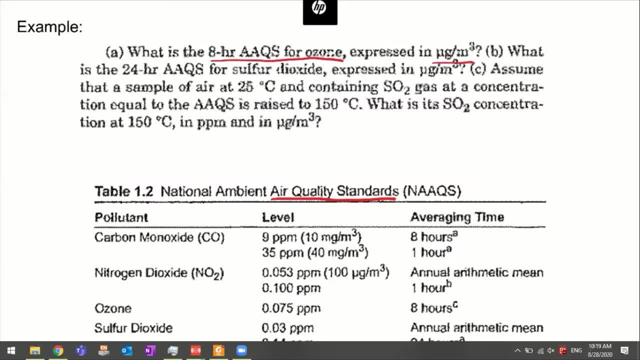 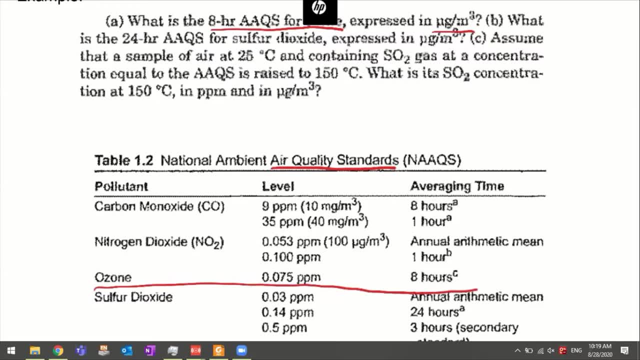 into ppm. Okay. So we've just got the number of micrograms per meter cube Okay. So if you check this table here for ozone, we have the 8-hour average Right, So it has a regulated level of 0.075.. 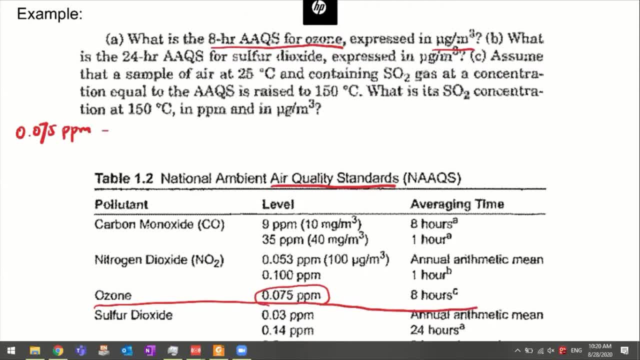 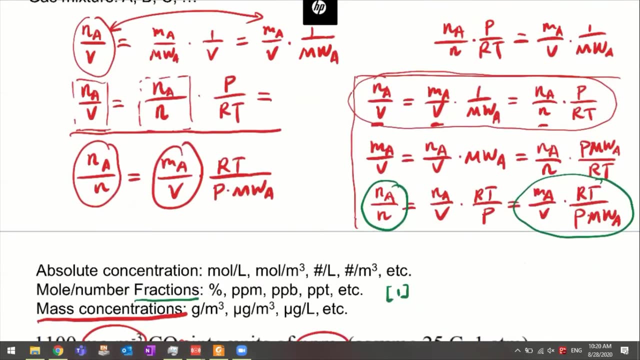 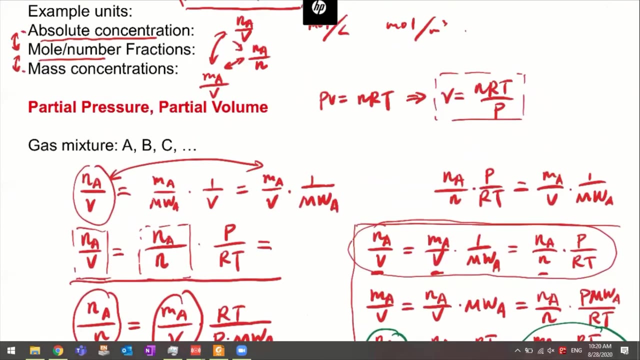 And let's try to convert this into mass concentration. Okay, So if you go back to the equation, which is the mass concentration equation, should we use, Let's say here: all right, So we have the mole fraction, but we're trying to solve. 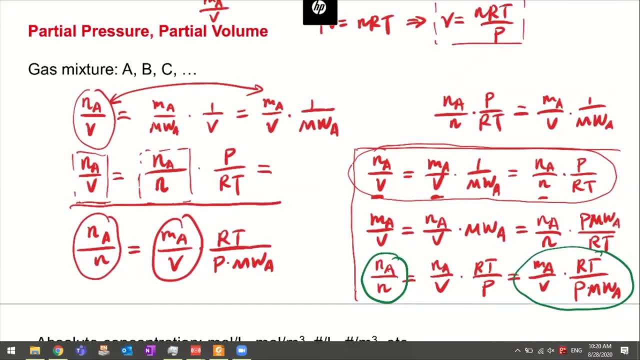 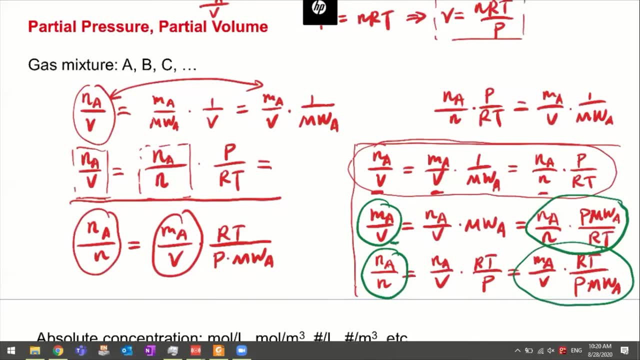 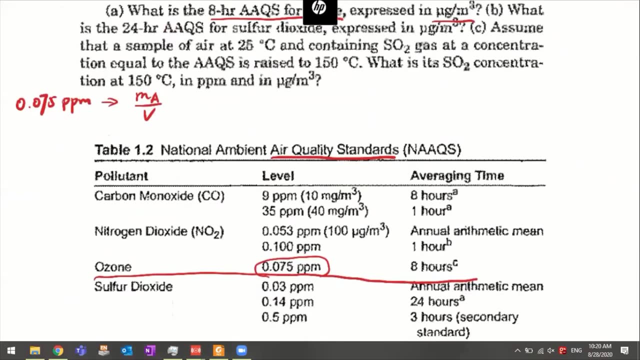 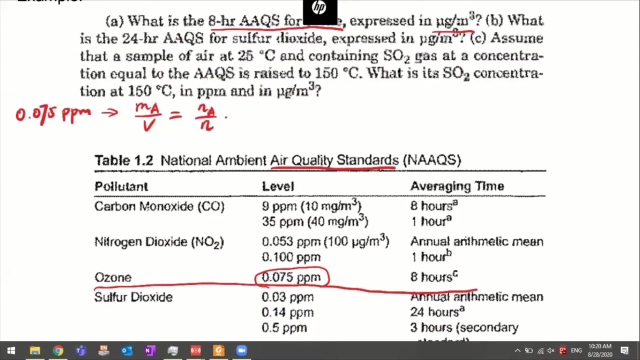 for mass concentration. we should use this one right Trying to solve for this mass concentration here. okay, So if we compare, then we know mass fraction should be equal to Na divided by n multiplied by P, weight of A divided by RT. 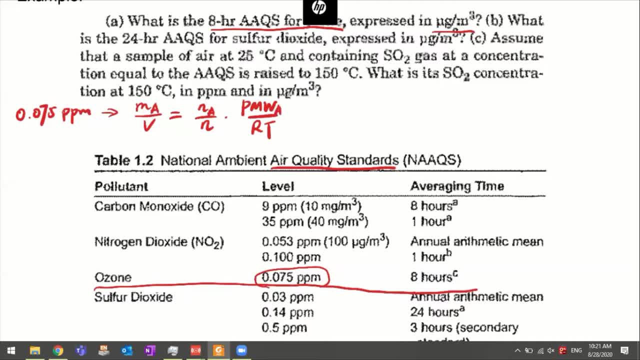 So in this case we just need to figure out what is the weight of this. Can we convert it to that mass, The weight, plug in all the numbers so we know that the mole fraction here is 0.075 ppm. so we need to multiply. 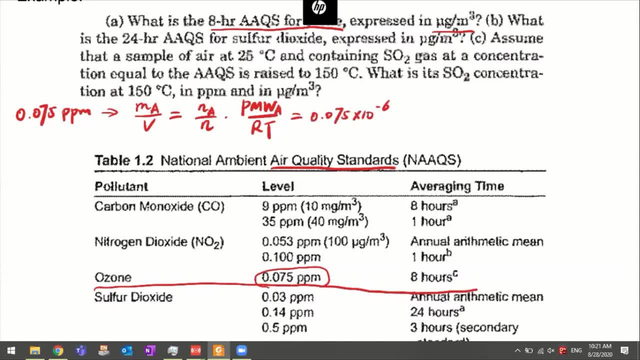 this mole fraction by 10 to the negative, 6, first, right, and then plug in all of the other numbers, we have pressure equal to 1.01, multiplied by 10 to the fifth, and then for the molecular weight of ozone, that's basically 03, right? we have 3 multiplied by 16, that's 48, but we shouldn't use. 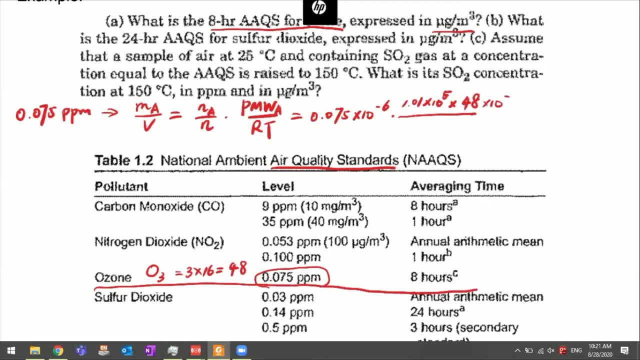 48 directly because we need to use standard units. okay, so 48 multiplied by 10 to the negative 3, we convert that into kilogram. and then r is equal to 8.314. multiplied by temperature: 298.15 kelvin. right? so if we plug in all of these numbers, i think i should also have the equations. 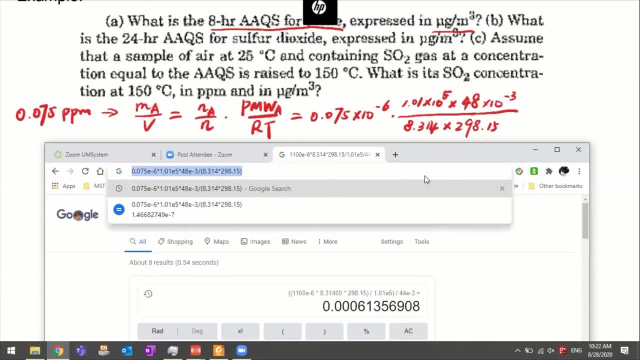 okay. so this is the equation that i put in: 0.075 multiplied by 10 to the negative 6, and then this pressure molecular weight of ozone divided by r and temperature. okay, what we get is 0.1. okay, so it's gonna be 1.47 multiplied by 10 to the negative 7 kilogram per meter cube. 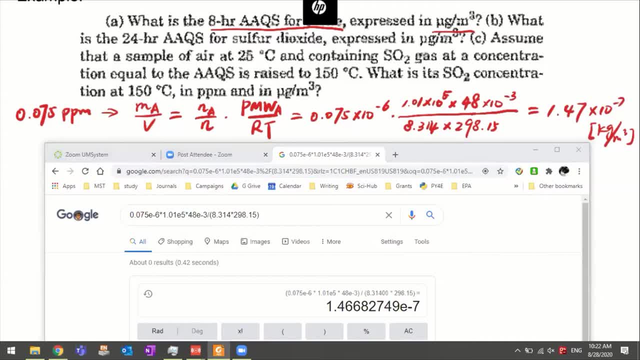 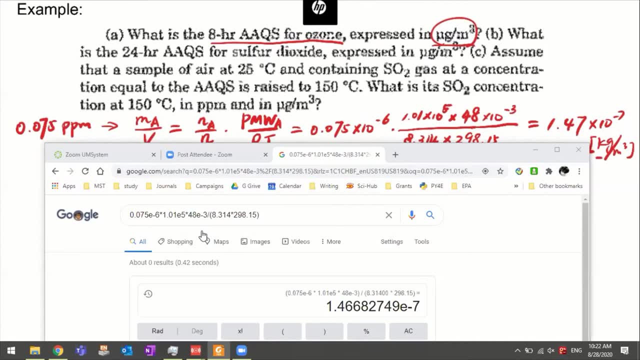 okay, so you see, this question asks you about the mass concentration in micrograms. okay, so we need to further convert this mass unit into micrograms, in that instead of using kilograms. So we know that 1 kilogram is 10 to the negative, 10 to the third power of grams. 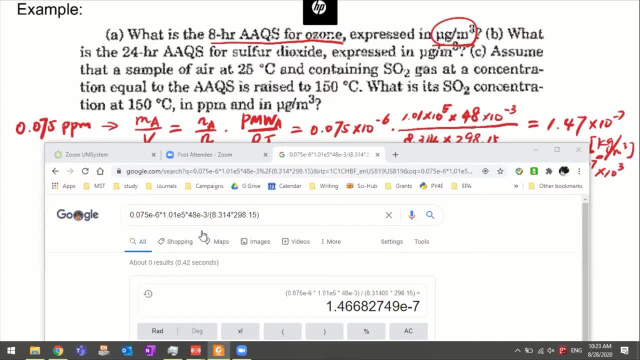 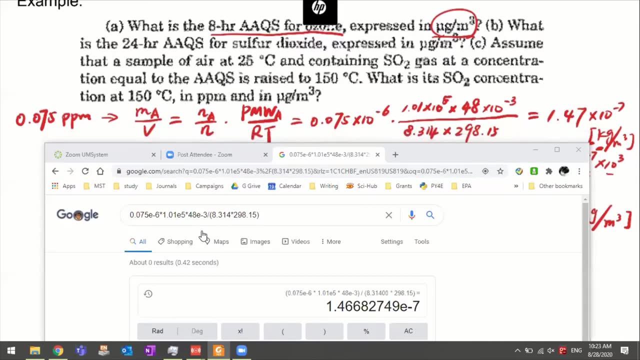 And if we want to convert grams into micrograms, that's another 10 to the sixth. So finally we should get 147 micrograms per meter cubed Here. we got 10 to the ninth, And then this is 10 to the negative 7.. 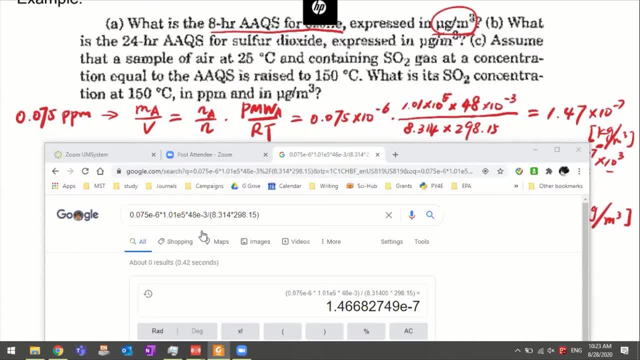 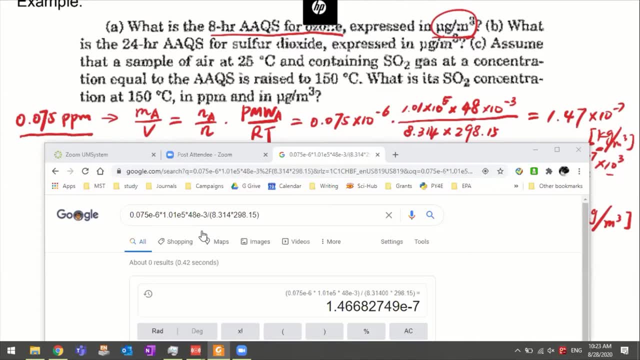 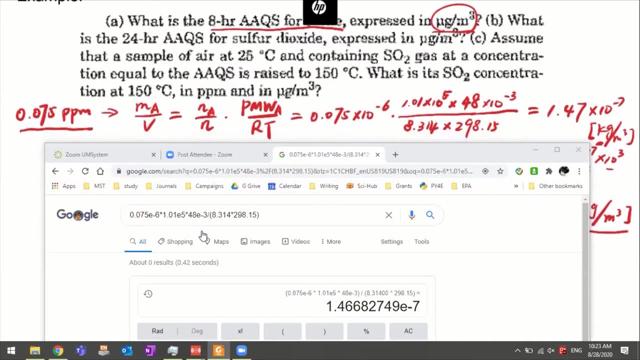 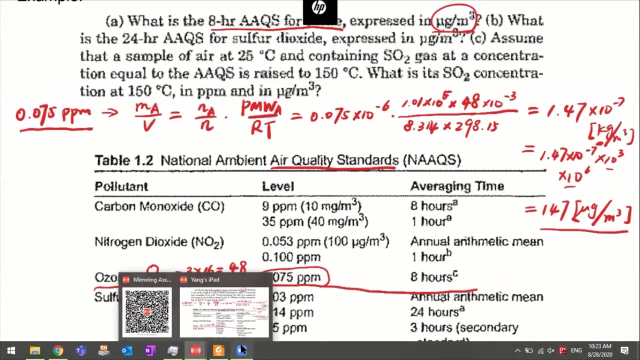 So we have 147.. So basically, this is how we can convert this number, fraction- into mass concentration. By using the equation we just showed, you can calculate what is mass concentration. So any questions until now, I mean, if not, we'll just continue. 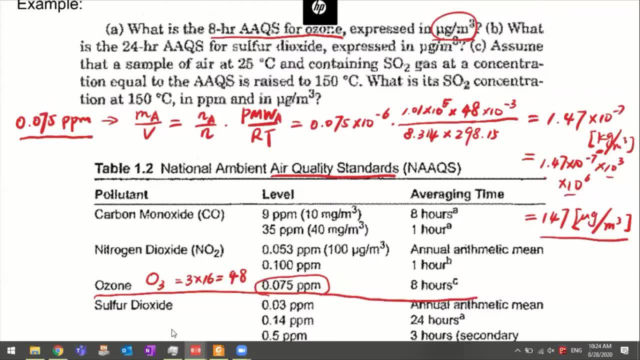 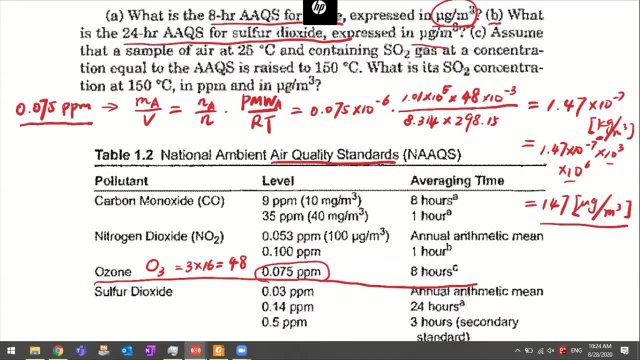 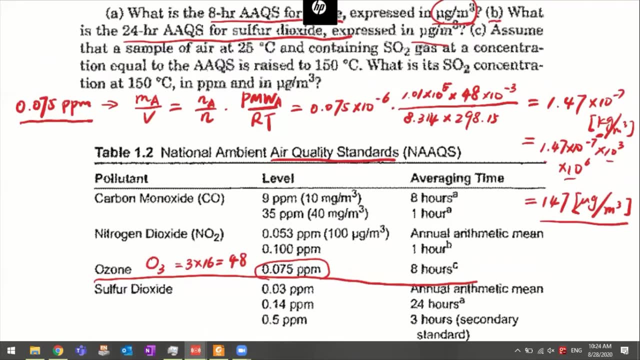 All right. So if we look at the problem B- so what is the 24-hour AAQS for sulfur dioxide expressed in microgram per meter cubed? Then if we look at the sulfur dioxide and also look at the 24-hour average, 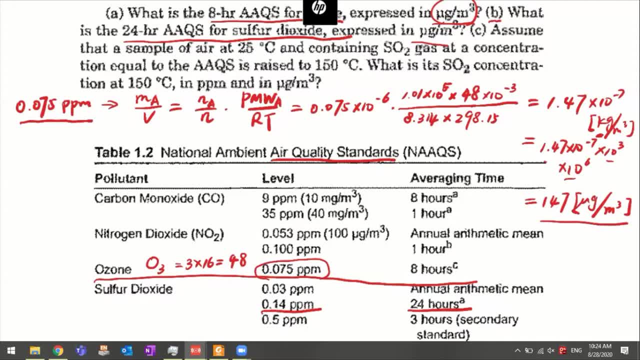 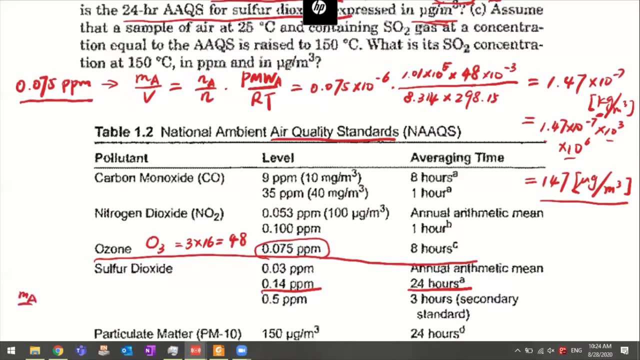 that's going to be 0.14 ppm, right? We need to convert this ppm into mass concentration again, So we should use a similar equation, except that the number we plug in will be different, right? So again, we should have MA divided by V equal to NA. 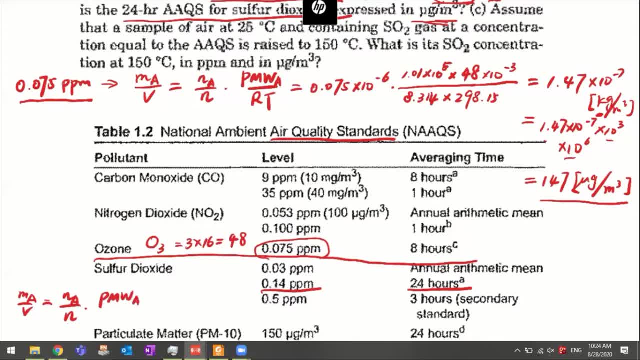 divided by N. p. molecular weight of A divided by RT, right. So the number fraction. here, instead of using this number, we're going to use 0.14 multiplied by 10 to the sixth, And then it's the same. 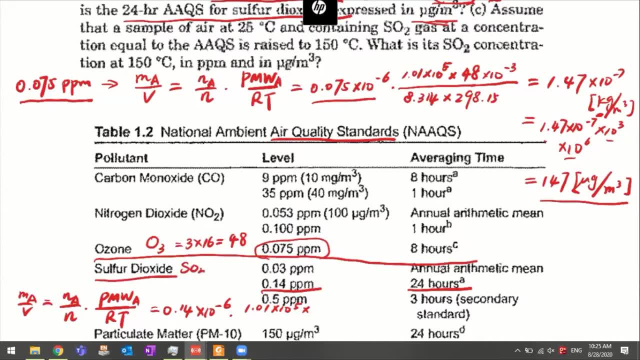 So the molecular weight of sulfur dioxide, that's 32 plus 16 multiplied by 2, which is 64 gram per mole, right? So we have 64 multiplied by 10 to the negative 3, divided by 8.314 and 298.15, OK. 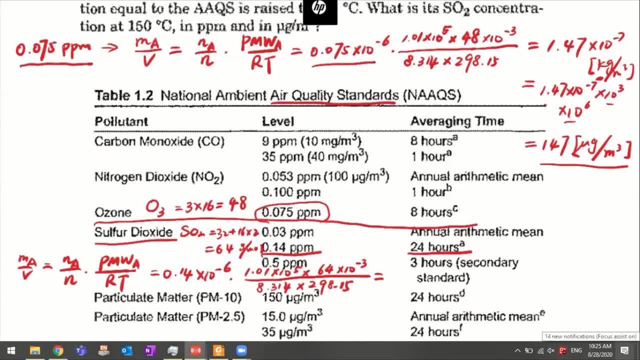 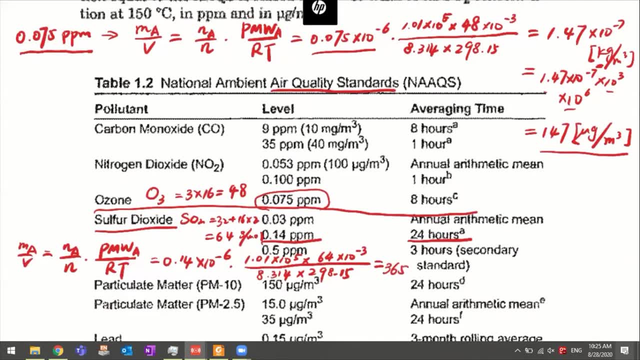 So, based on this equation, we can calculate. OK, So, based on this equation, we can calculate out what is the mass concentration And if you have time to do the calculation, that's going to be 365 microgram per meter cubed. OK, 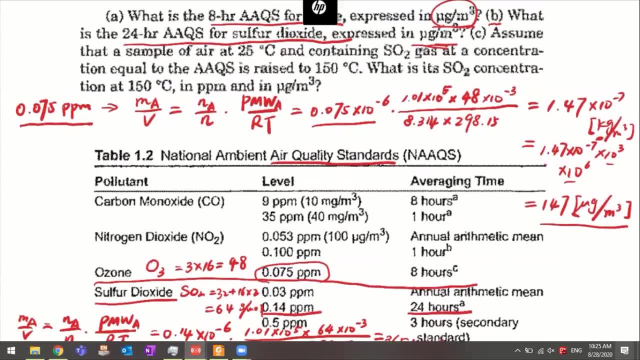 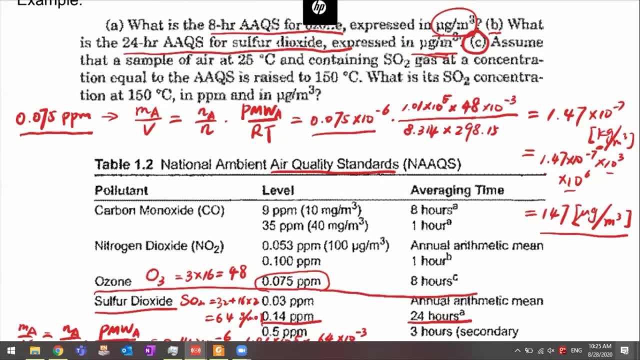 So this is how we can use these equations to convert the units. OK, So now we look at the third question. This is actually a quite interesting one, all right, So assume that there is an air sample at 25 Celsius And it contains the sulfur dioxide gas. 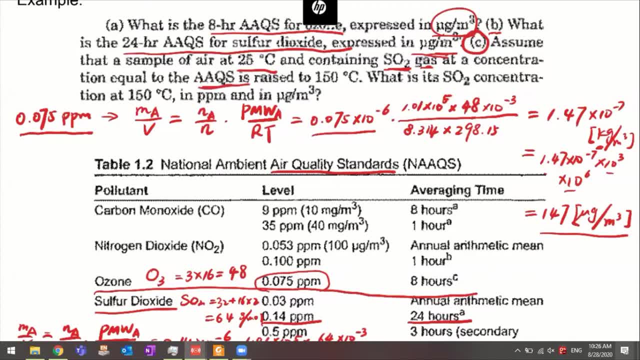 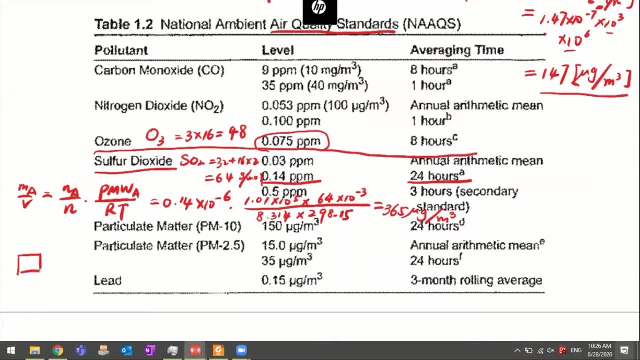 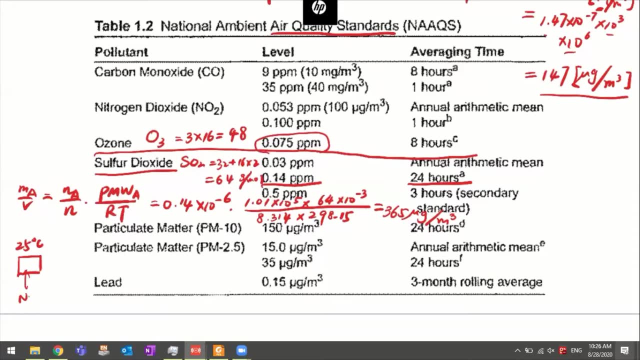 at a concentration that's equal to AAQS. OK, So let's assume that we have a gas mixture, Let's say we got a bag of air right, And then that's collected at 25 Celsius. And there are some. of course there are nitrogen and oxygen. 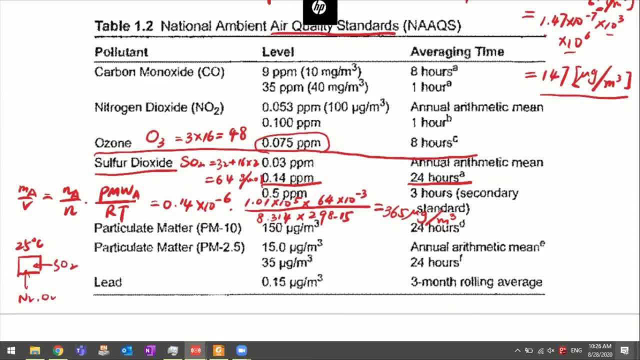 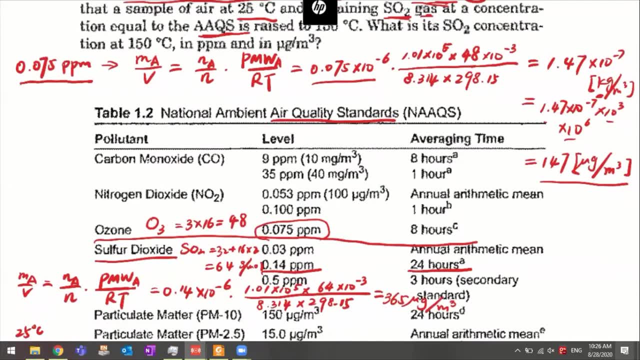 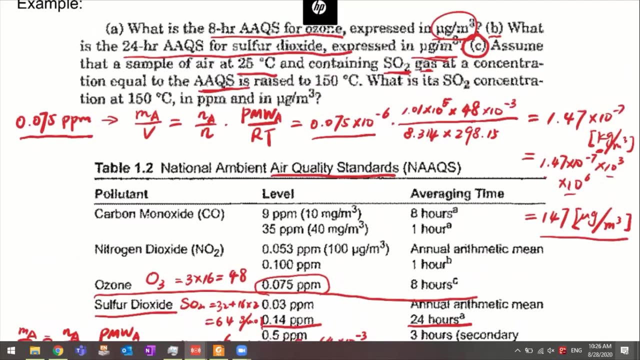 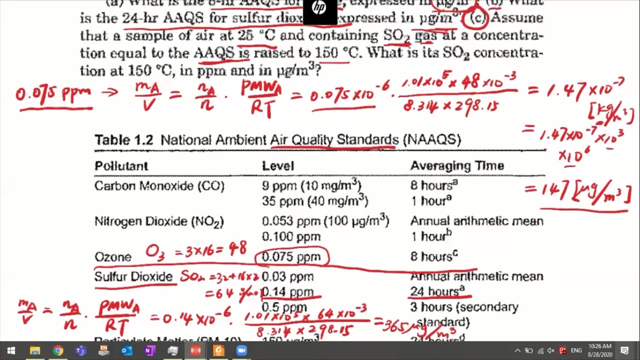 But there are some sulfur dioxide And the sulfur dioxide concentration is equal to the AAQS. OK, So we can calculate out the mass at this temperature, which is 0.14 ppm. So now we decide to heat it up, So we decide to raise its temperature to 150 Celsius. 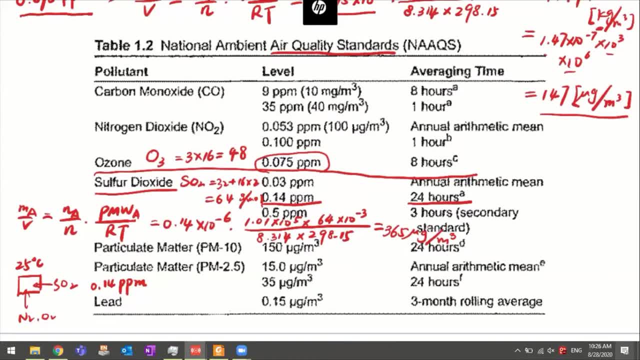 So what we know is that if it absorbs heat, basically if the temperature raises, then the volume will also expand, right? Originally we have a small volume, But since we heat it up, now it has a larger volume. So we ask: about what is the sulfur dioxide concentration? 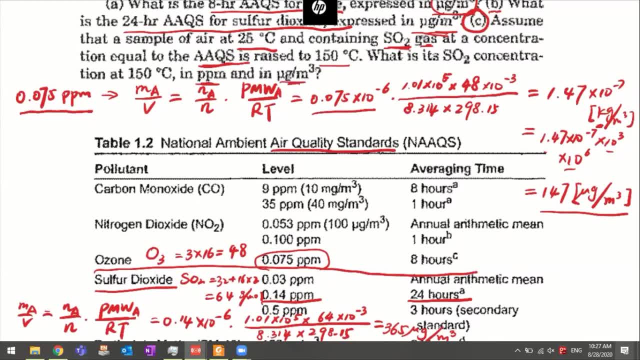 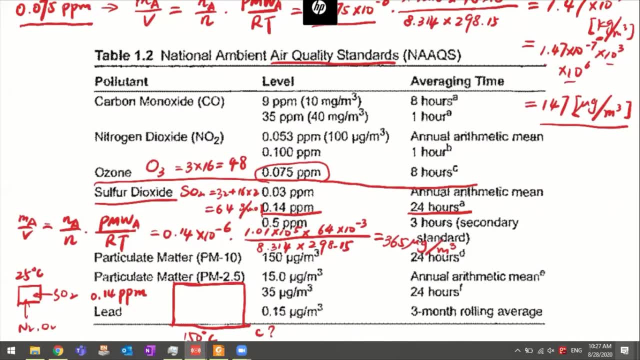 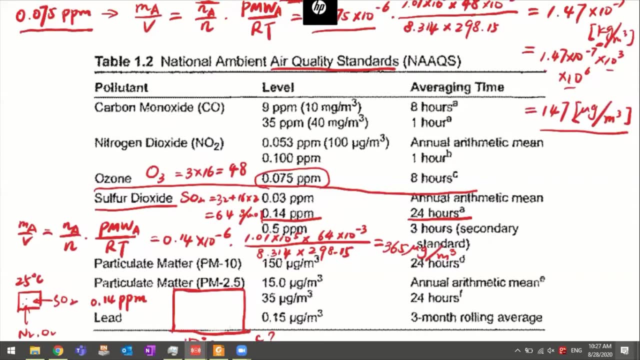 in ppm and in microgram per meter cubed. OK, So basically it wants us to solve for the concentration in both the number fraction and mass concentration. So one thing we know is that let's say for the gas mixture in the beginning we're going to need: 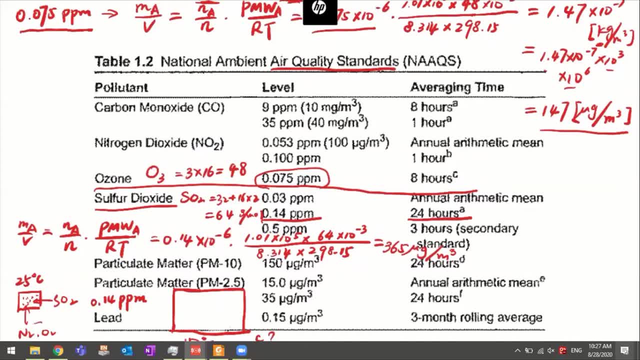 we know that there are a certain number of nitrogen and oxygen inside, But also the number of the sulfur dioxide is also fixed inside, right. So if we decide to heat it up, so the actual number of these gas molecules will not change, right. 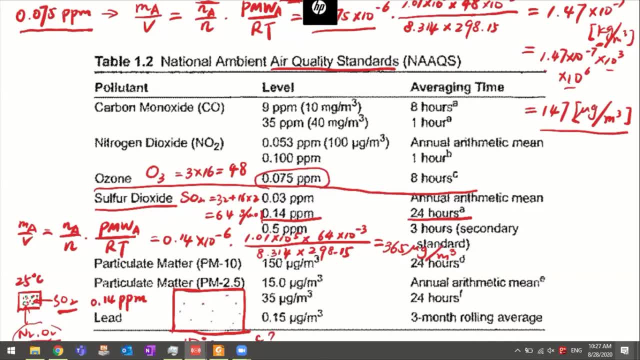 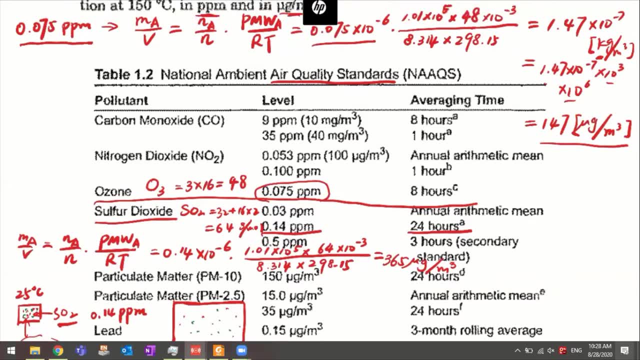 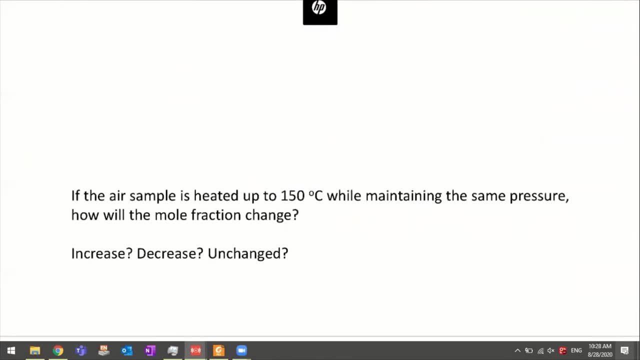 It's just that their distance becomes longer, right? So instead of very crowded here, their distance will become farther, OK, So if that's the case, how will the mole fraction change? OK, Is it going to increase, decrease or end change? 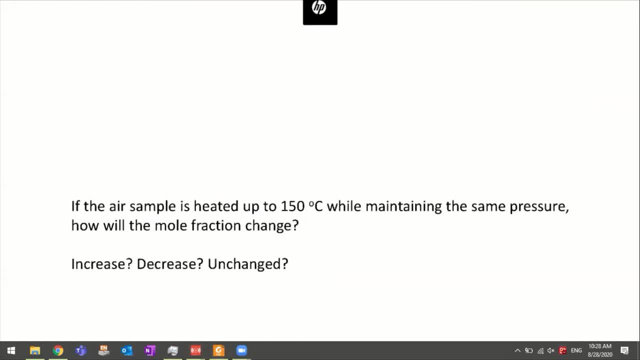 So we'll do another pool. So if the air sample is heated up from 25 to 150 Celsius while maintaining the same pressure, how will the mole fraction change If we consider that, basically, it's just the air getting more diluted? 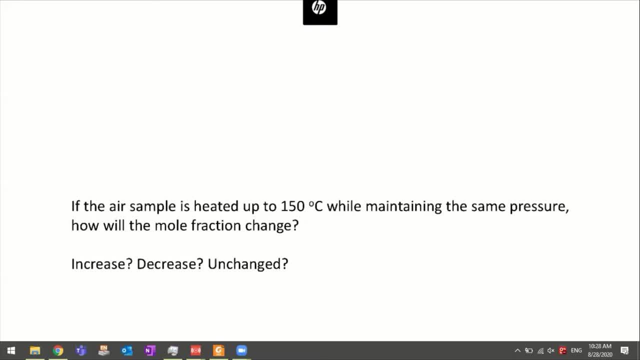 We're going to move to the next step, which is to add all of these things in to the reaction. So we're going to add a little bit of nitrogen to the fraction. So we're going to add a little bit of nitrogen to the fraction. 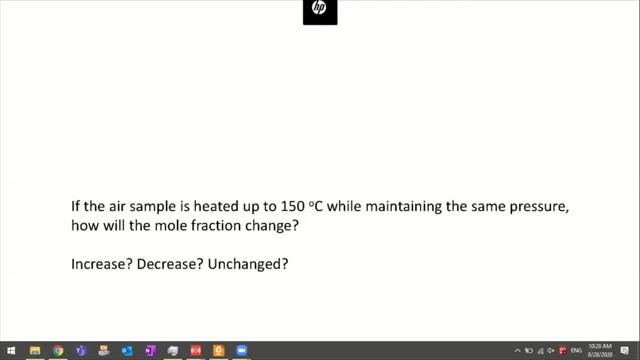 And then we're going to add the nitrogen to the fraction. Okay, I'll just stop here. I think I probably didn't explain this system very well, So let's see the results. It should be the same, unchanged. Okay, should be the third one. I know that. 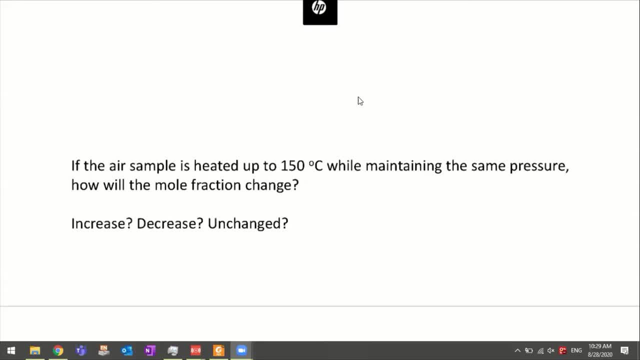 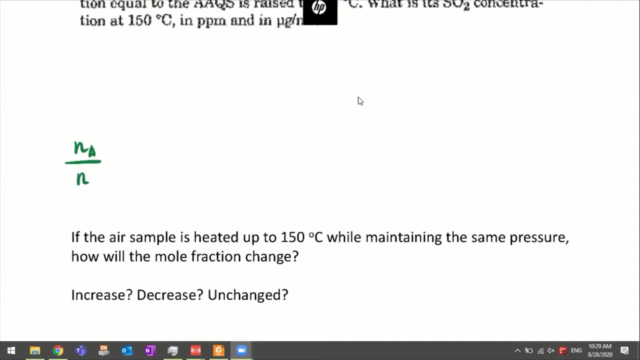 some of you might think that once we dilute something, the concentration should decrease. But that concentration is not the mole fraction. The mole fraction is basically the number of moles for this species divided by the number of moles for all the gas species. So while 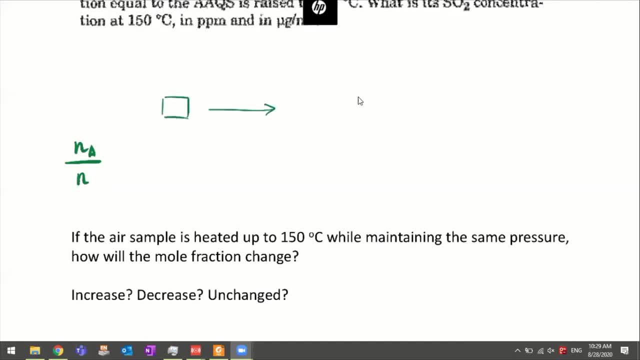 the sulfur dioxide is getting diluted into a larger volume. the other gas species are also getting diluted, Right? And because this is a sealed system, 150 Celsius. so let's say there were 10 molecules of oxygen or nitrogen in the beginning and just one molecule of sulfur dioxide. So if 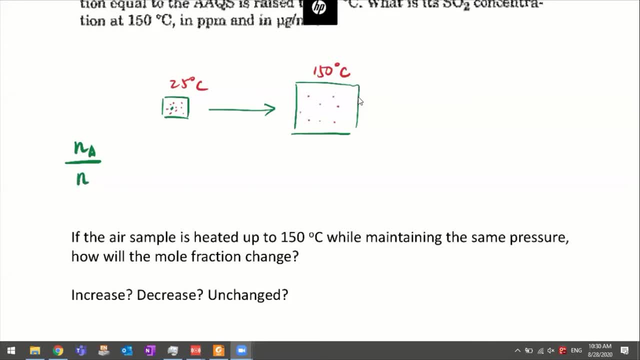 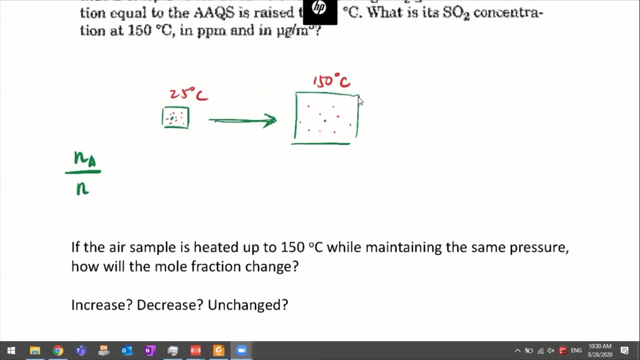 we heat it up, the number of molecules for the nitrogen or oxygen are still the same, And it also applies for the sulfur dioxide. So basically, the number of moles for all the different species were unchanged. It doesn't matter if we heat it up or shrink it right, And because of that the mole fraction should. 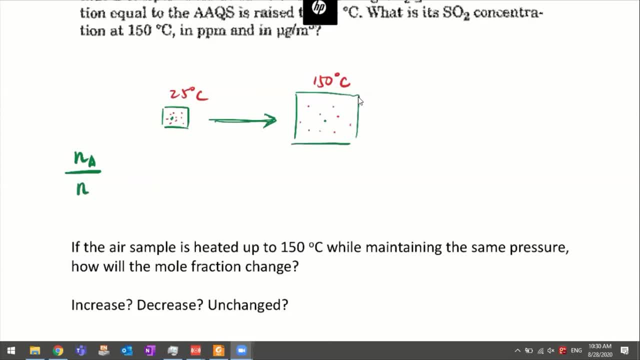 be the same. All right, So does that make sense? Right? So if you think that makes sense, you can show a sum up. Okay, Okay, All right, Yeah, So basically, that's why the mole fraction should be unchanged, right? And then, if we 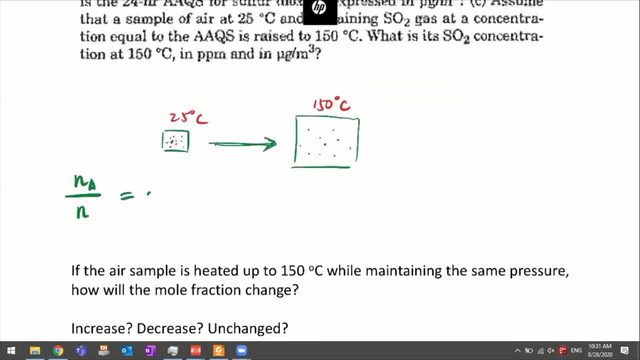 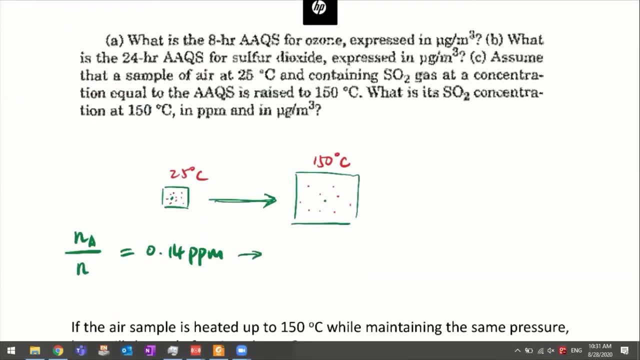 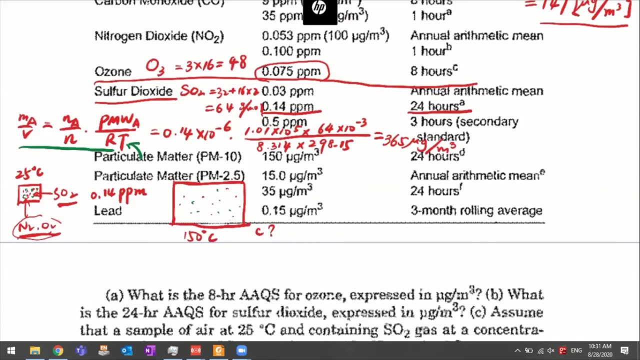 know that mole fraction is unchanged. we know that the mole fraction is still 0.14 ppm. right, We just need to convert this into mass concentration. So we're going to use the same equation here. except for that, the temperature We're going to need to plug in 150 Celsius. 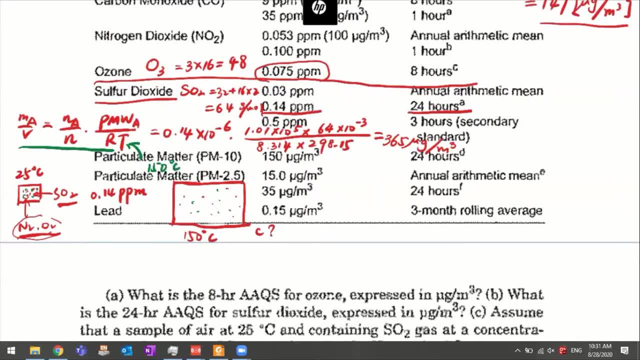 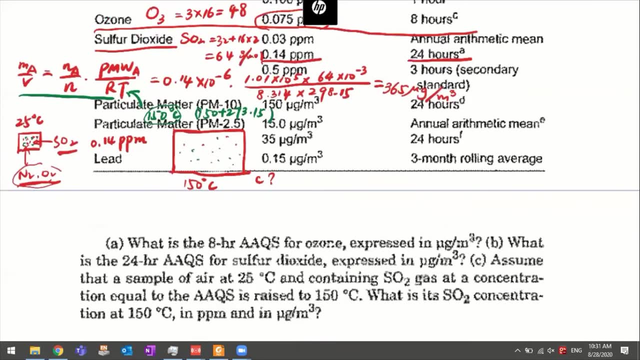 But we're not going to directly use this value here because we need to convert that into Kelvin. So that's going to be 150 plus 273.15,. okay, So you can find out that the actual answer should be the answer. final answer should. 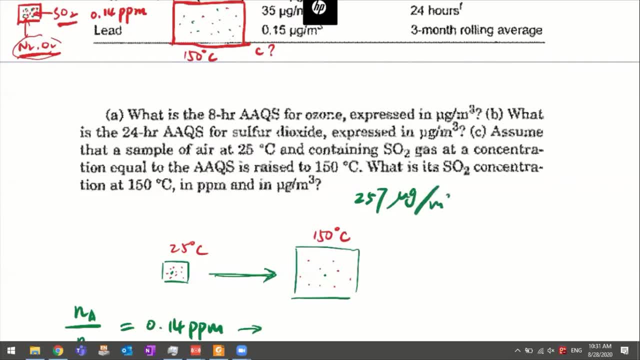 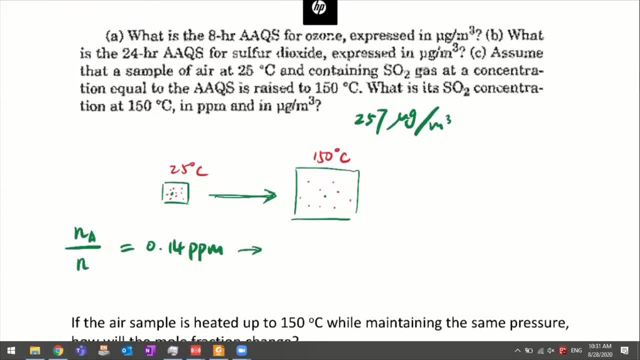 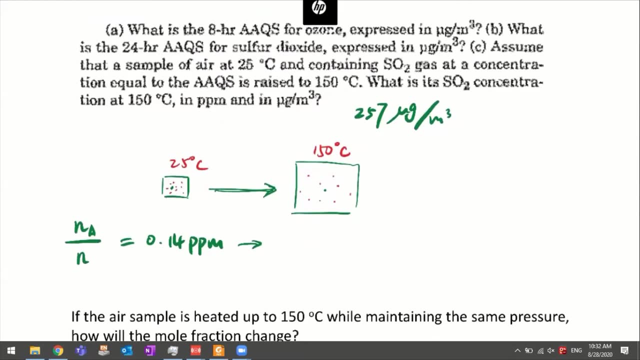 be 257 microgram per meter cube. okay, So I know that, um, these are a lot of calculations, but we have to go through this process because we're going to use that quite a lot later in our class, Although not related, not very related to the particular matter, but when we're talking. 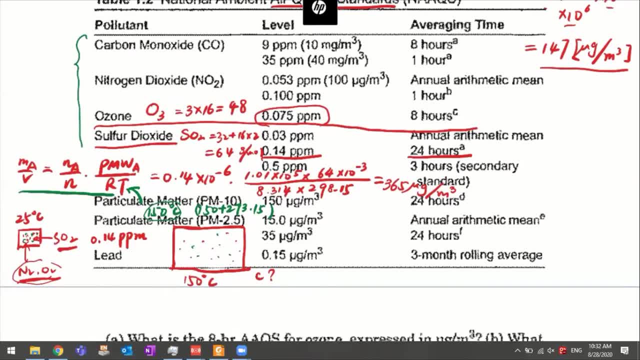 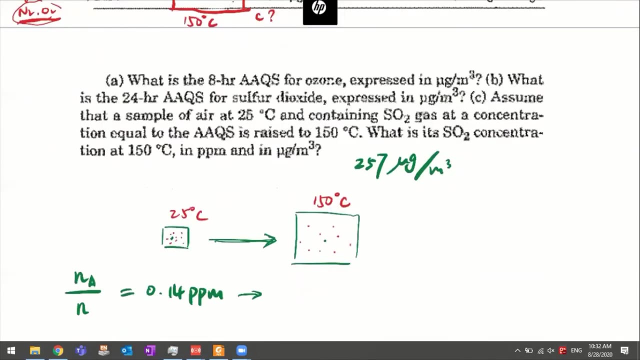 about the control of all of these gas pollutants. So basically, carbon monoxide, nitrogen dioxide, ozone and sulfur dioxide will go through a lot, a lot of these unit derivation. Okay, So if you have any questions, just let me know. and, um, um, I have to say maybe this: 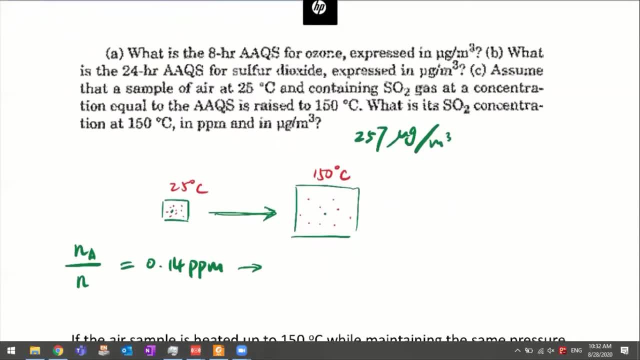 is still too early, but uh, so unit conversion is going to be a part of the exam. okay, So maybe not directly doing these calculations, but maybe as a part of the um problem when we're trying to solve for a larger problem there. 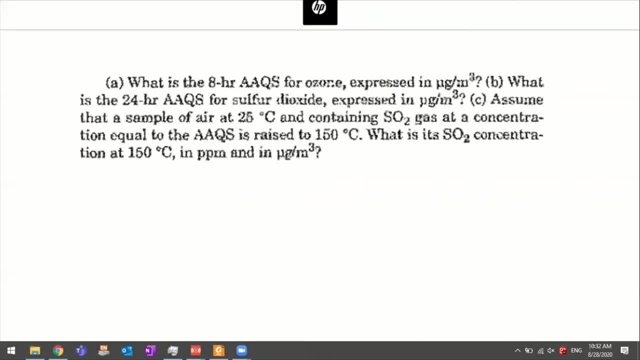 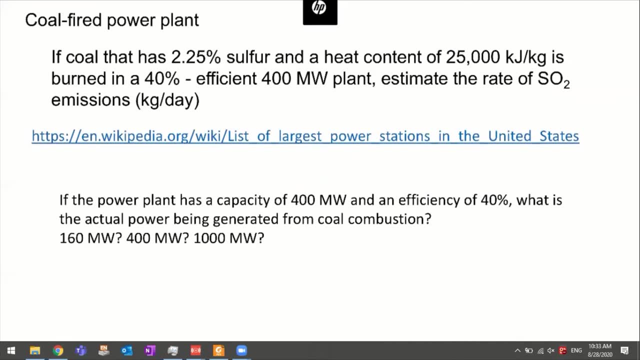 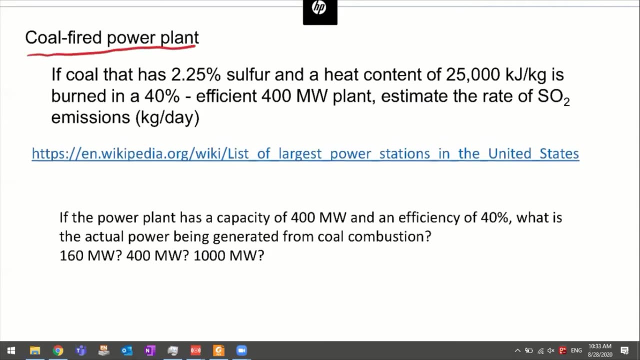 Okay, So we went through this. Okay, So we went through these problems already. And finally, this is the last part of calculation I want to show in this class, So we're going to talk about this: uh, coal-fired power plant- quite a lot. 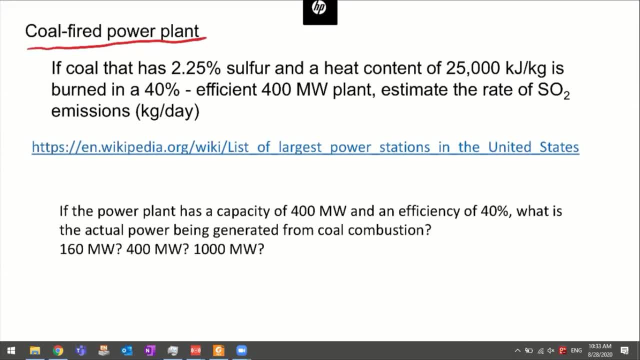 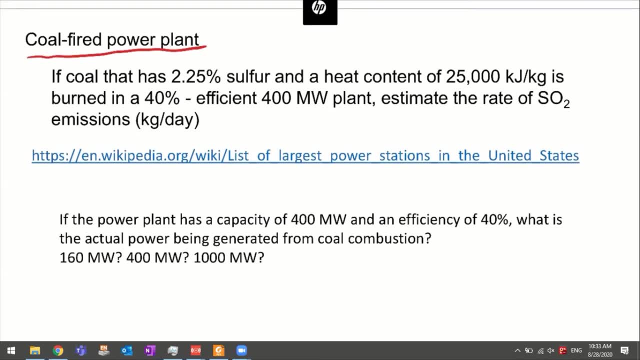 Okay, Um, also, we'll discuss the project. The project is going to be related to, uh um, the pollution control for a coal-fired power plant. So here there's. this is uh uh, quite complicated, Okay. 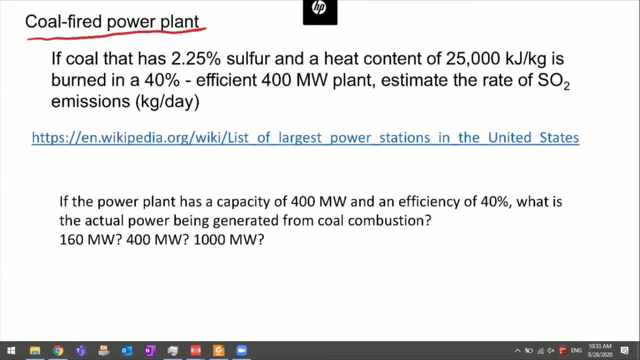 This is a quite common question we're going to deal with. So let's say, if the coal we decide to burn has a sulfur content of 2.25% and a heat content of 25,000 kilojoules per kilogram, okay, 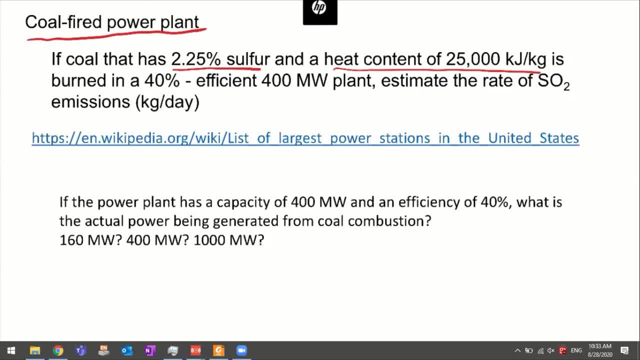 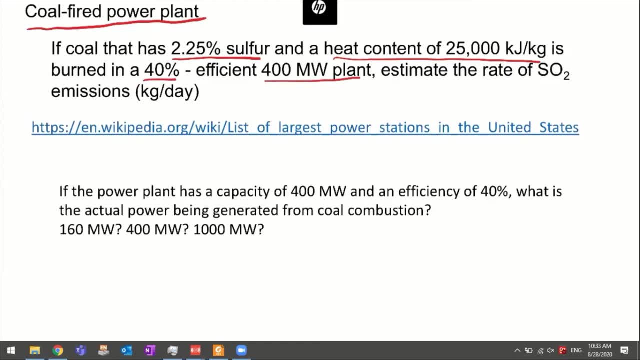 So let's say this is coal we're using and it's being burned at a 40% efficient, 400 megawatt power plant. Uh, it wants us to estimate. what is the rate of? uh, Uh, Uh, Uh. 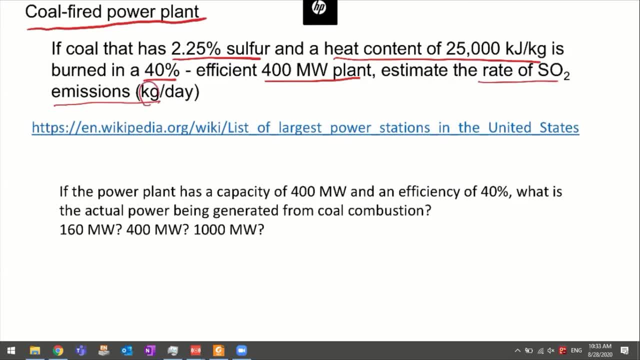 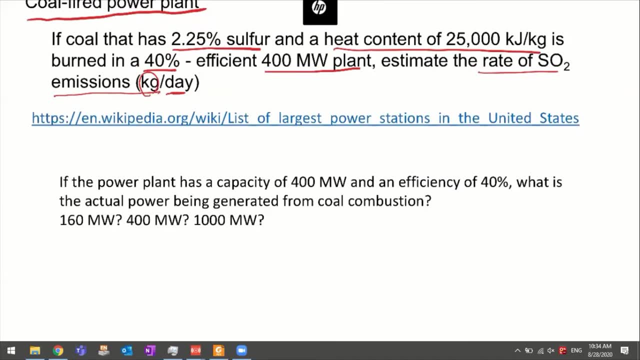 The rate of uh sulfur dioxide emission. Okay, So what is the emission of sulfur dioxide per kilogram per day? Okay, So how do we approach this problem? Um so, first we need to know how a coal-fired power plant works, or how it burns the coal. 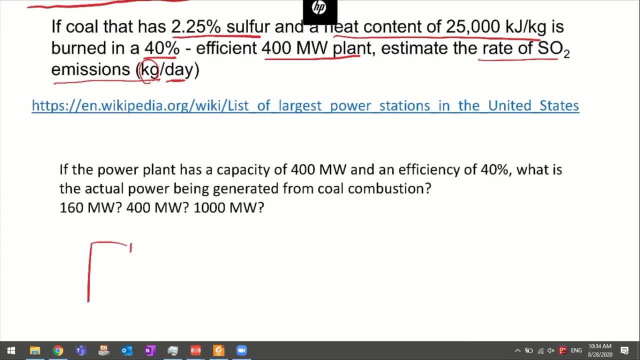 So let's say, um, this is our coal-fired power plant. Okay, So this is normally how a combustor works, right? We have a mesh that has a lot of coal in here, Right, a lot of flame, and in the coal combustor there are pipes. that contains water. you? 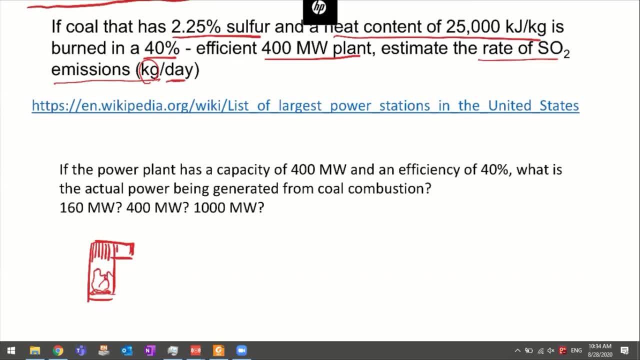 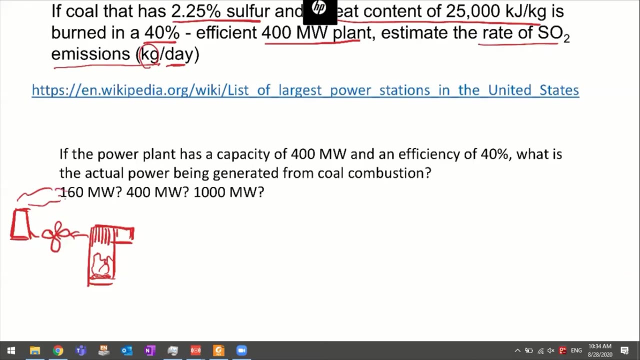 know that the coal-fired power plant use the steams to run the turbines, right? so all of these water get boiled up, right, go through the steam, go through the steam, right. finally, it goes to the cooling tower. so that's basically the really large towers we saw when we pass by a power plant, right? so basically this. 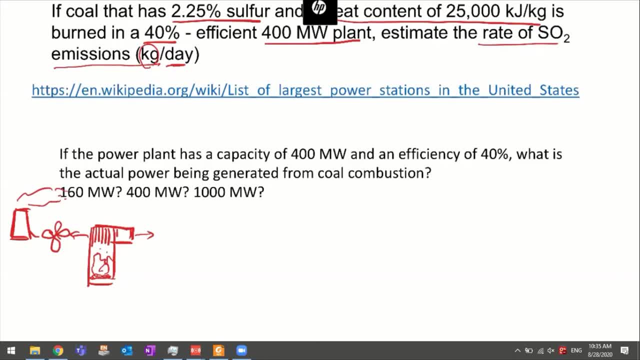 is a water site, but on the other hand, when we burn the coal, we generate a lot of particles or gas species, right? so here we have a series of, let's say, particle control devices. right, we call this cyclone, and we also go through like a electrostatic precipitator. 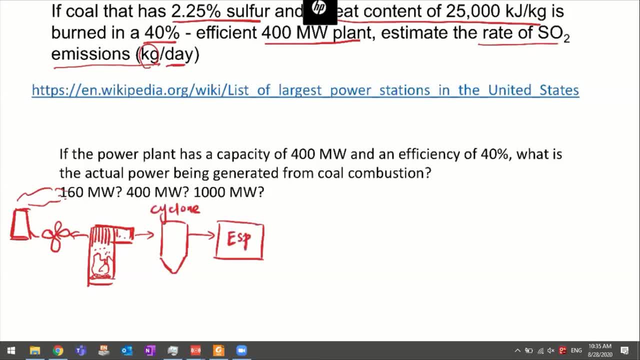 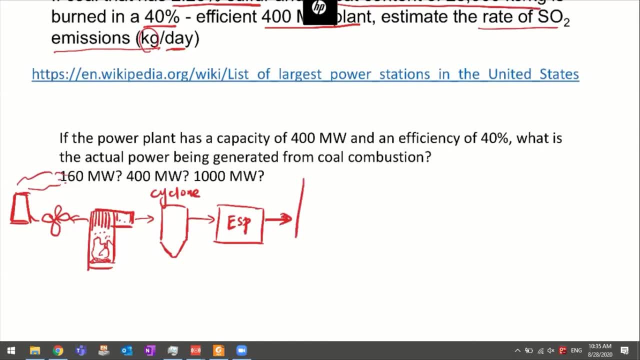 so I'll just write these names out. we'll get to learn more about these devices later on in the semester, okay, and then finally, it's going to be sent to a stack, okay, so that's why, when we go by power plants, we'll see those cooling towers. 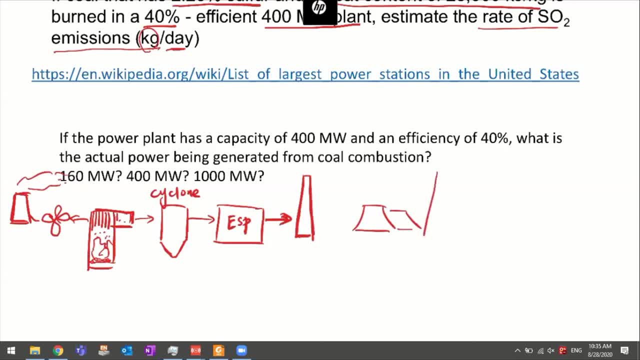 which are relatively shorter, and then we're going to see really high stacks. okay, the stacks emits all of these pollutants to the air, but the cooling tower just emits the water vapor. so the cooling tower not necessarily generate any pollution here, it's mainly the stacks here. okay, so let's say this: 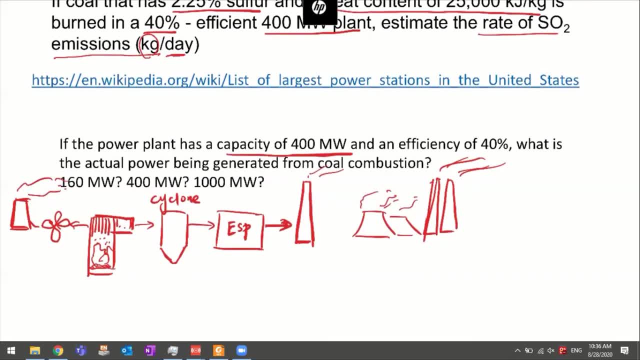 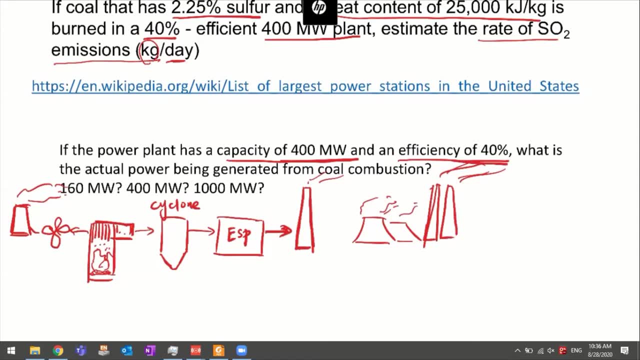 problem tells us: if the power plant has a capacity of 400 megawatt and also it has an efficiency of 40%, okay, so then what is the actual power being generated from coal combustion? because we know power is coming from coal combustion and it has an efficiency of 40%. so, finally, the coal-fired power plant has a. 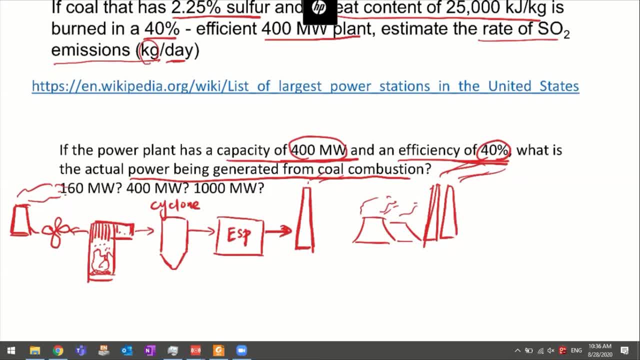 capacity of 400 megawatt. so then we need to calculate what is the actual power, what is the entire energy that's coming from the coal combustion? okay, so this is a quite basic question, right, let's do some calculations here. so which one should it be? 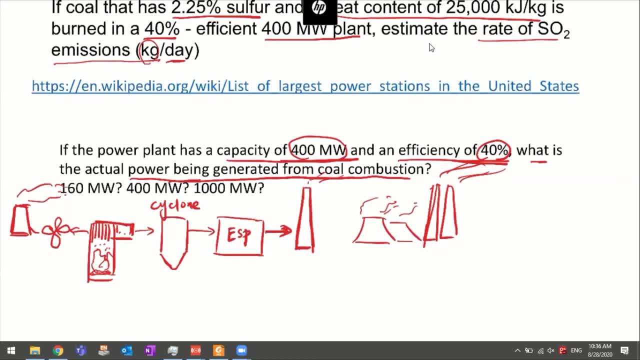 you choose. okay, we'll stop here. so, unfortunately, this time adjusting the answers in the hands of fewer people, so it should be 1000 megawatts this time. right, we look at this at this far. so here's another example by in river hotel. so if you just have a power plant, 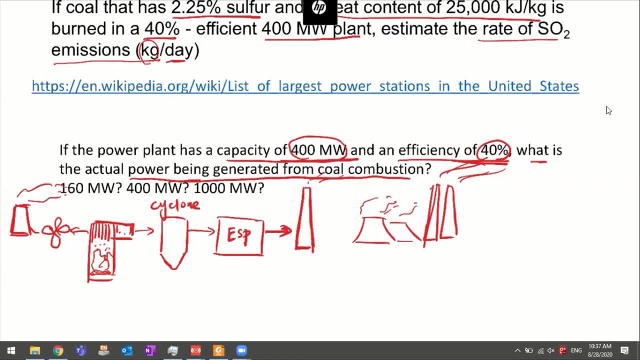 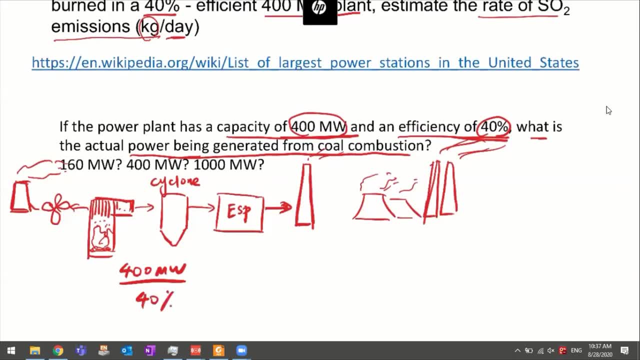 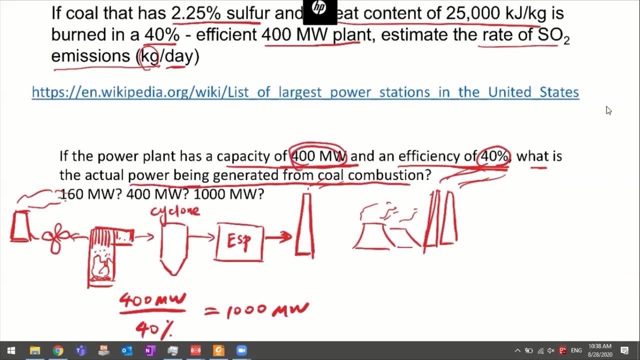 watt. okay, the rationale is we need to divide 400 megawatt by 40%, so you can think of this problem in this way. so let's say we have a power plant of that has a capacity of 400 megawatt, so this is what the power plant tells to the 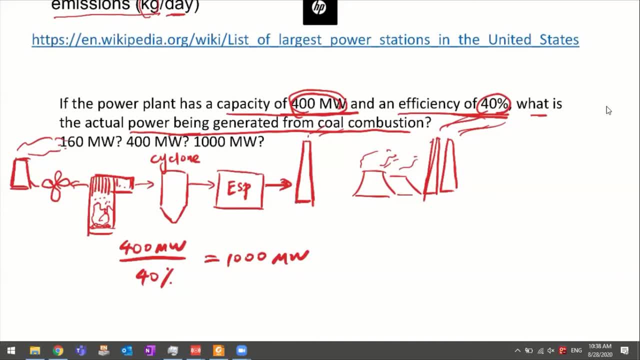 public. okay, this is this amount of electricity I'm generating or providing to the community. so 400 megawatt means what? so it means megajoules per second. right watt is joule per second, so this is the energy that's being sent to all. 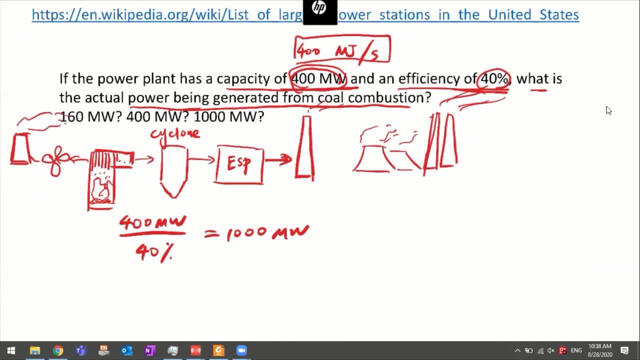 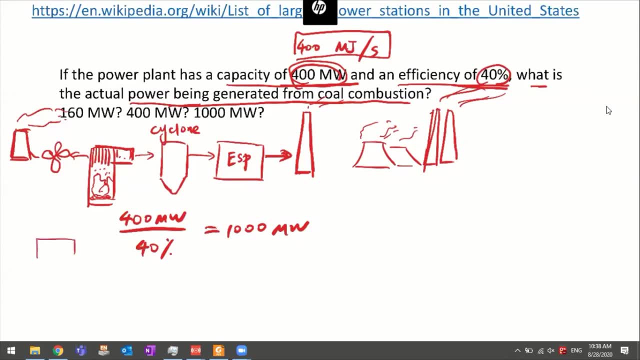 the different households. so let's think of this co-combustion problem as the, as the process. when we're using gasdoll- right, so we know that at home we normally boil water inside. okay, so it's either using gas or using electricity, right, and so, in terms of this process, 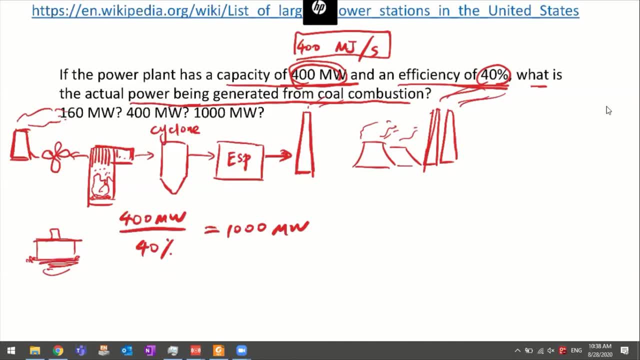 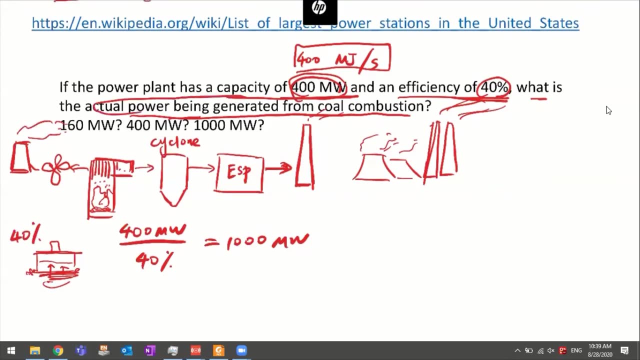 there have to be an efficiency. it's not not all of these heat are being transferred into the water inside right, so there's an efficiency and for this problem we have an efficiency of 40%. so if you try to know what is the actual power being generated or what is the what, what is the actual power being? 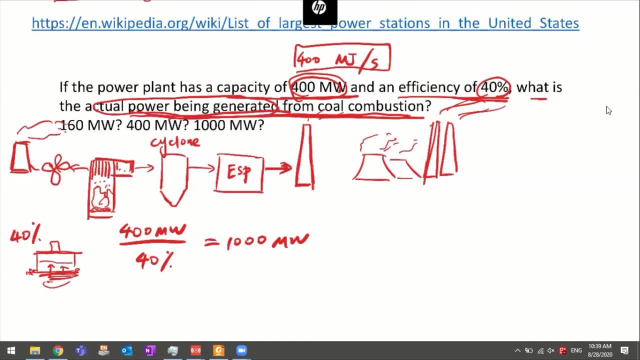 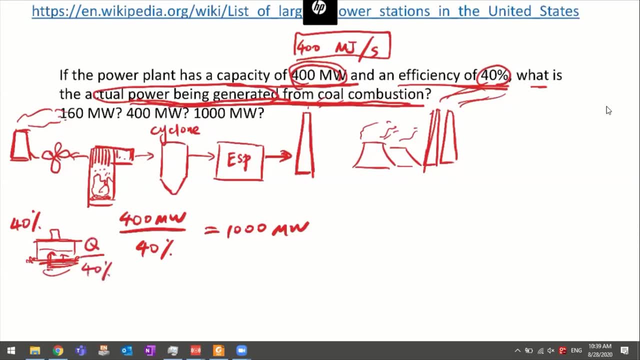 generated from co-combustion. what is the heat being generated? from co-combustion or from this heating process? we need to use this energy divided by 40%, so this is going to be the actual power that's being used right, and because there's an efficiency, we can just generate a. 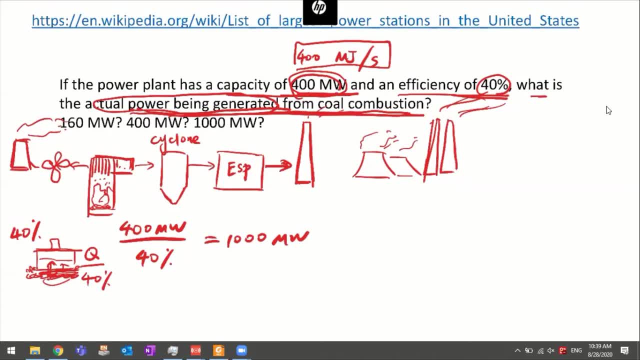 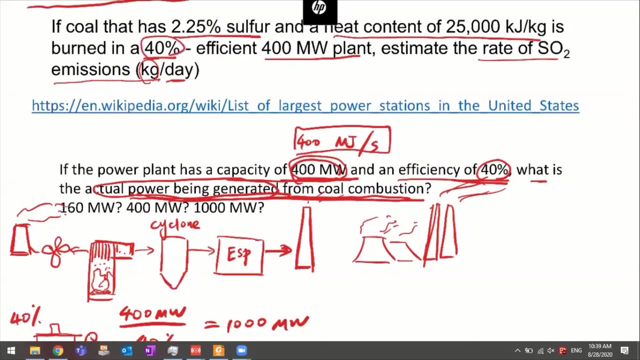 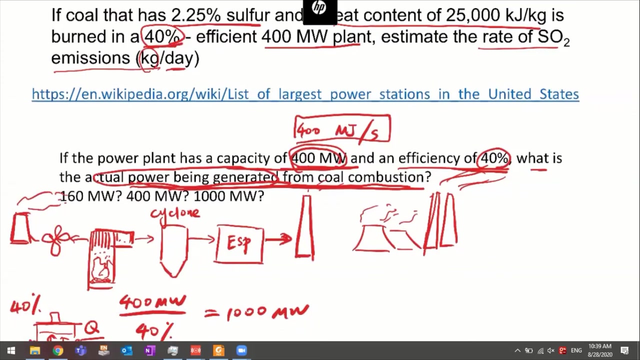 certain fraction of them, which is 400 megawatt. so does that make sense? right? so this is how the efficiency works. we're talking about these on power conversion problems, right? so if it has an efficiency of 40%, we're just going to divide this actual power of the, this process, by this efficiency. 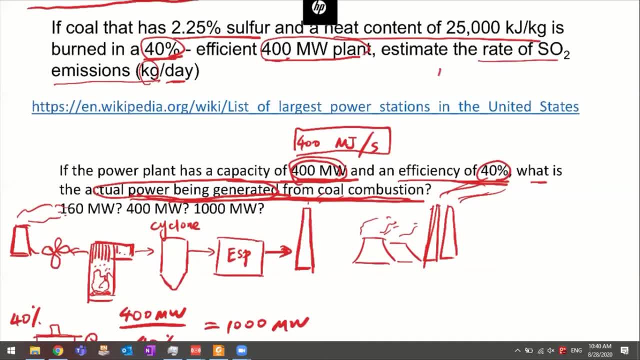 right. so let's say, if the co-combustion is generating 100 Joules of the power and the has a forty percent efficiency, the co-combustion gain is source: 2010 Joules of the power and it has a forty percent efficiency. 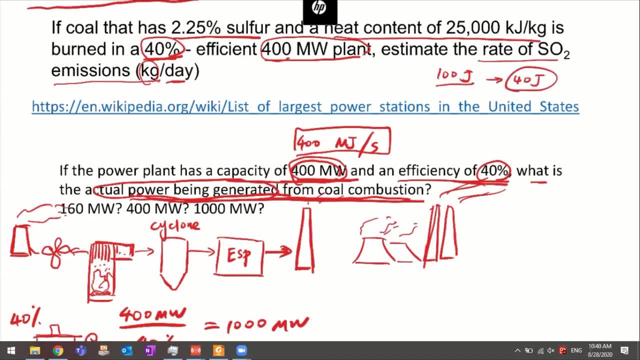 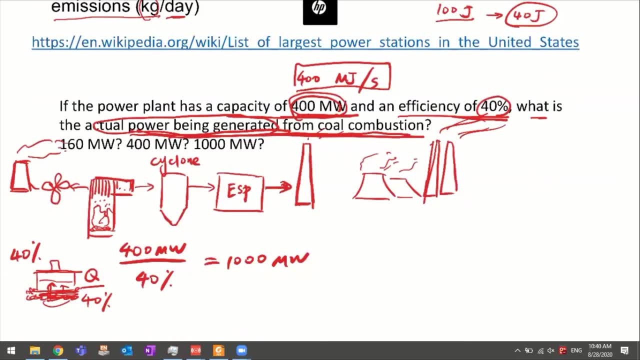 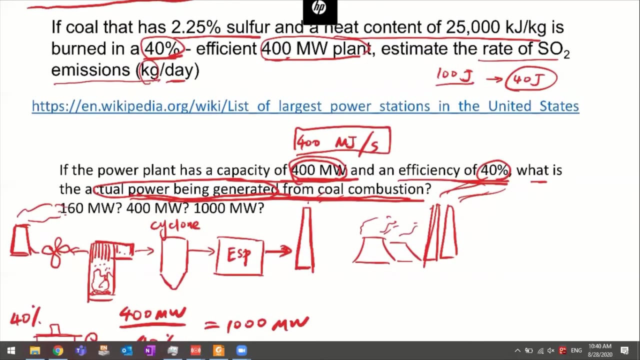 わか image. then it just means that 40 joules are being used to warm up the water. okay, so still confusing, or good, okay? um so you'll go through more practice on this problem. it's maybe a little bit difficult to understand in the beginning, but um so. 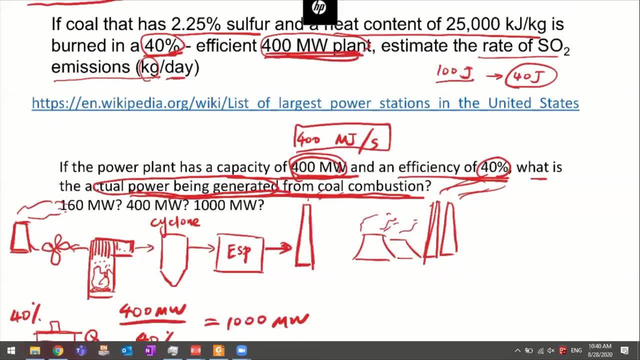 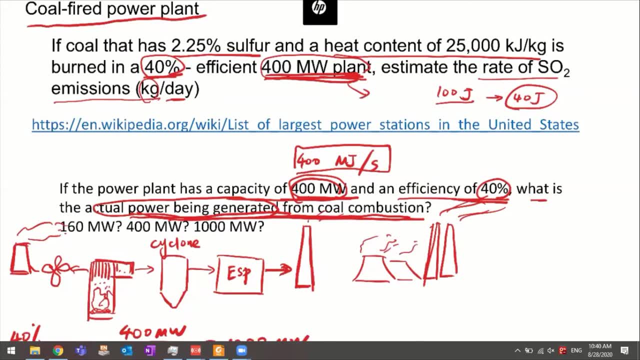 basically this power, what it stays for the power plant, it is just the um, the energy that uh, it transfers to all the different households. but there is an efficiency. when we're trying to obtain the all of these energy right, we're losing a lot of losing a lot of heat, losing a lot of energy when we transfer. 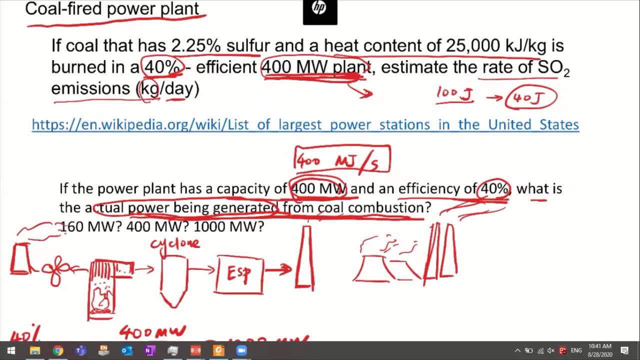 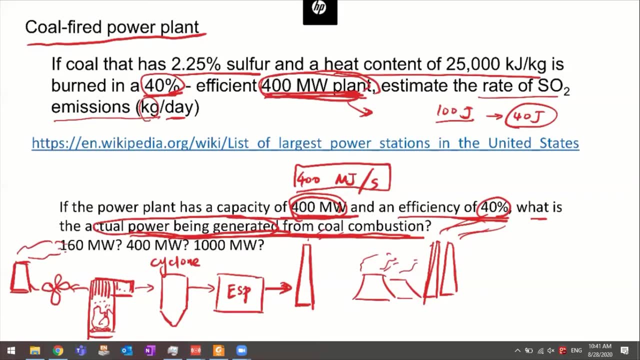 the heat into the electricity. okay, all right, so so, um, for this problem, we're also, uh, learning a term which is the capacity of a power plant. so this one, we're actually dealing with a smaller power plant here. so, uh, if you're interested, you can also. 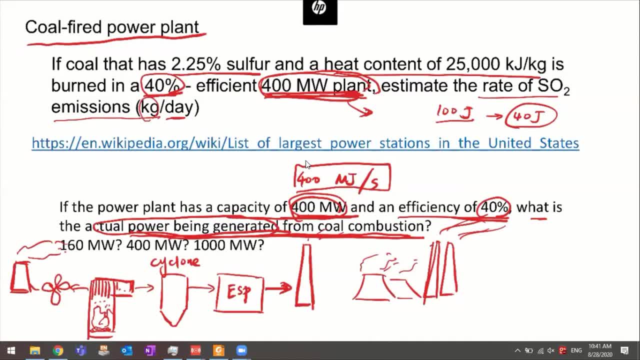 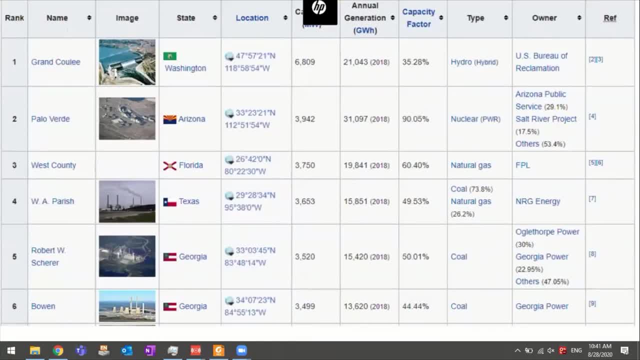 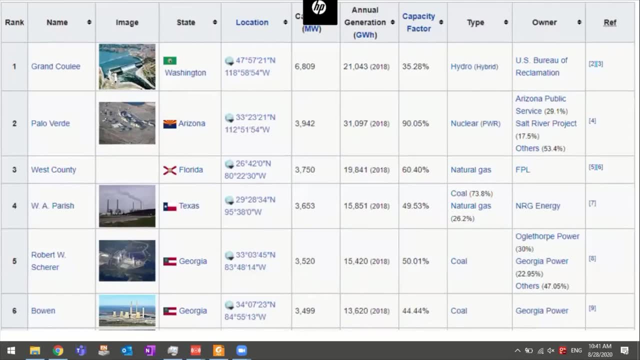 go through this link to look at what are the actual capacities for typical power plants in the us. so here i'm just listing out the top six power plants that we have in the united states. okay, So the first one. actually, it has a capacity of more than 6,000 megawatts. 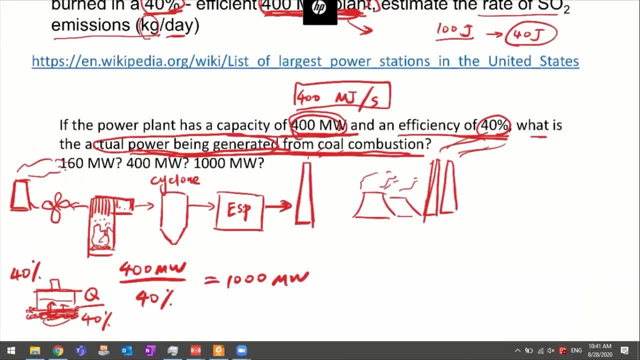 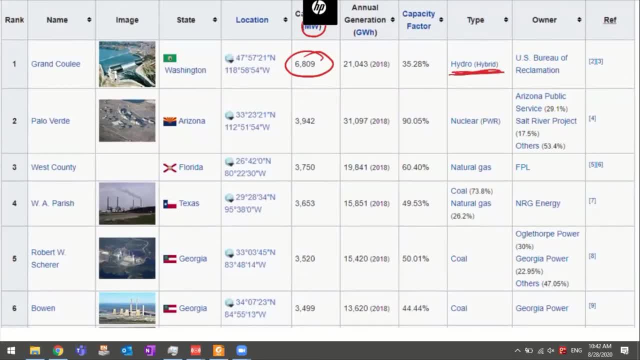 So it will be around, let's say, 15 of these coal-fired power plants, But this one is actually using hydropower here. But if you browse through, let's say among these top 100, actually most of them burns coal. 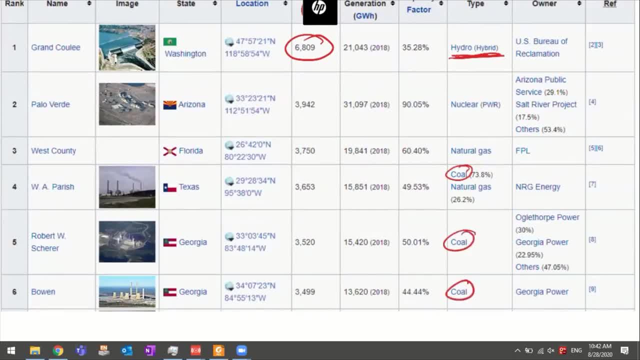 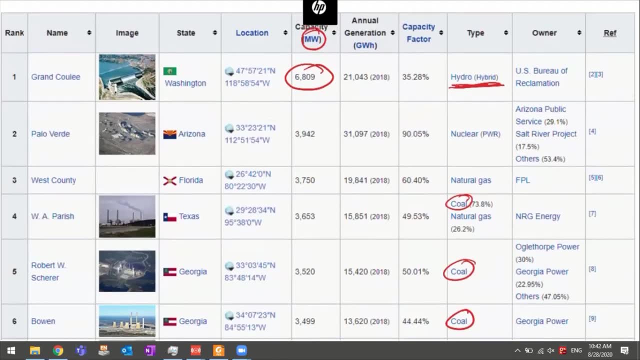 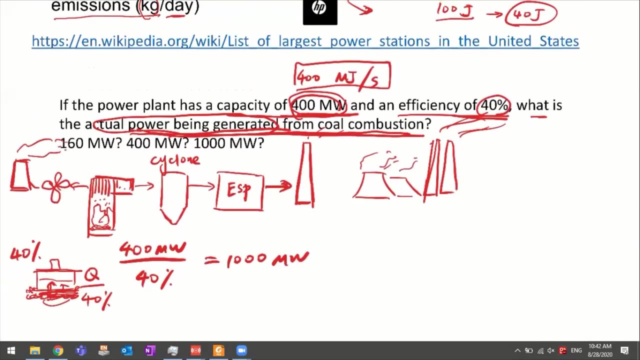 So here the fourth, fifth and sixth use coal to generate this electricity. So because of that, we need to consider what is efficiency. Basically, we need to burn more coal to generate this certain amount of capacity here Right. So for the sixth one, you see that the capacity is still. 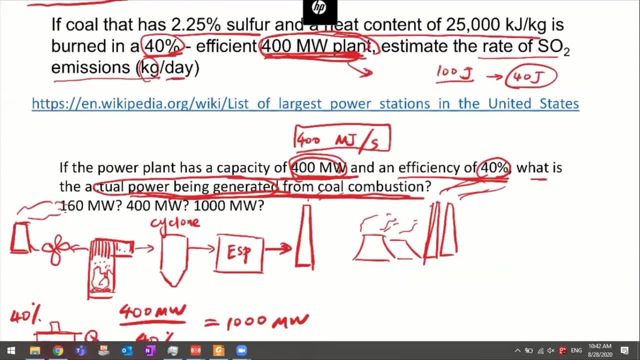 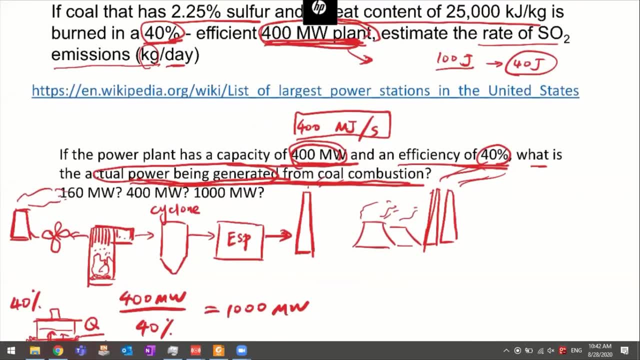 very high compared to our problem here. OK, So for this problem we have to generate more coal. For this problem. now let's try to understand how we can solve it. So first it gives us the capacity of this power plant. 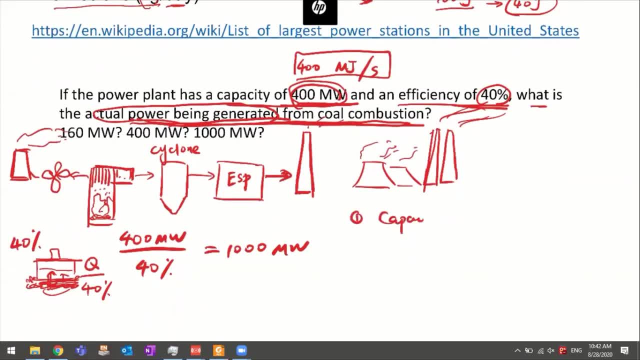 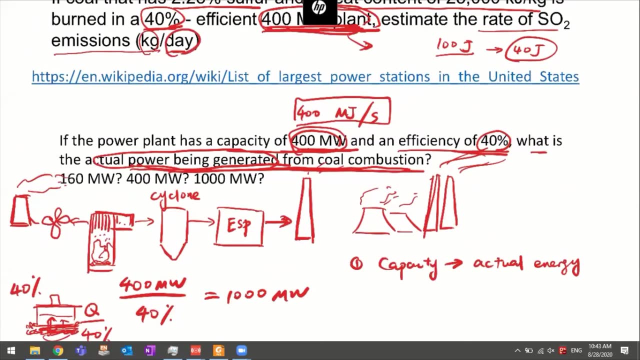 So, based on the capacity, we can calculate what is the actual energy being generated. OK, So this is talking about the energy in a day, right? So we need to first calculate the energy Right now. this is watts. Watts is per second. 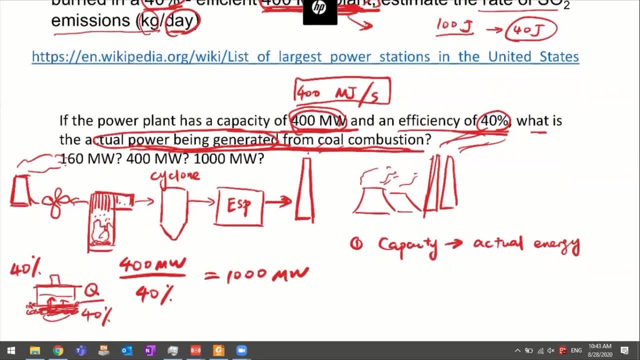 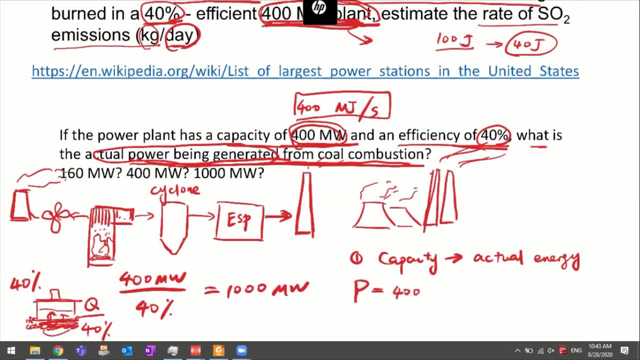 Right. We need to convert or need to calculate the energy for a whole day. So the energy should be equal to 400 megawatt. That's 10 to the sixth Right. So watt is joule per second Right. 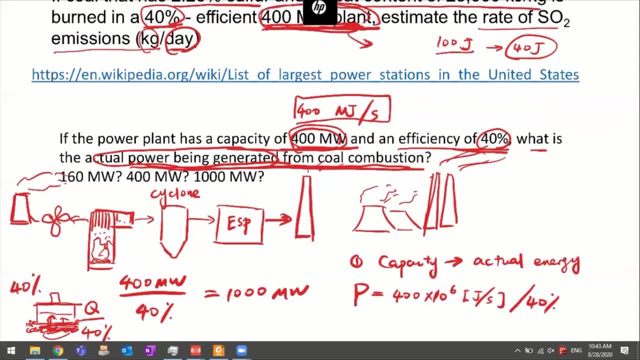 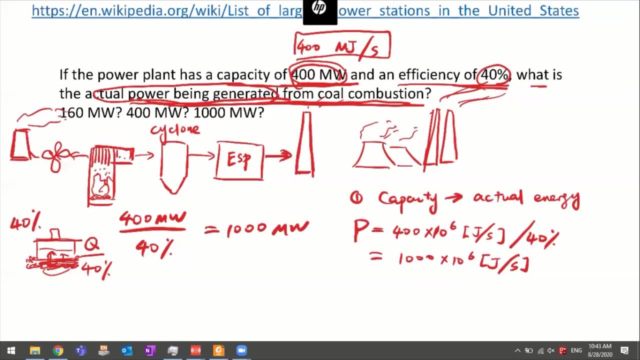 So we need to first divide that by 40%. That's going to be 1,000 multiplied. That's going to be 1,000 multiplied by 10, to the sixth joule per second Right. So in a whole day we need to multiply this p by 24 hours and 3,600 seconds. 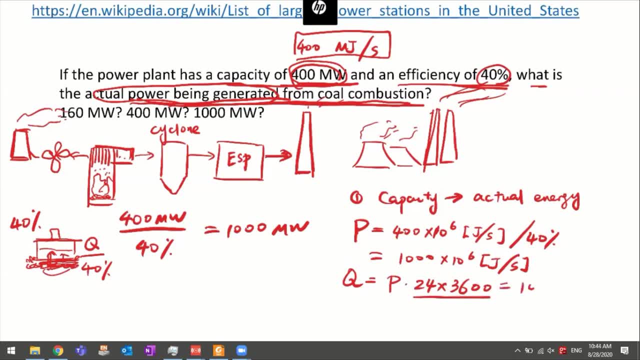 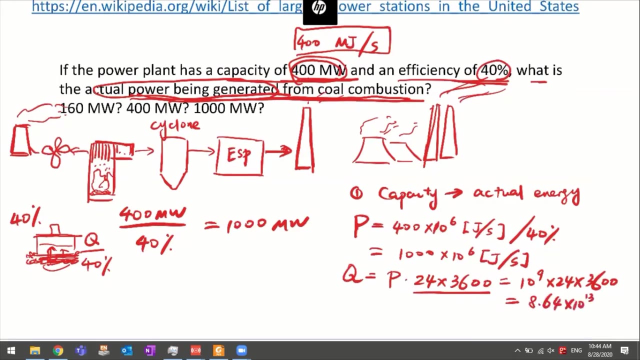 Right, This is talking about an entire day, Right? So that's going to be 10 to the ninth multiplied by 24, and 3,600.. So we're going to have, yeah, so we're going to have, 8.64 multiplied by 10 to the 13 joules. 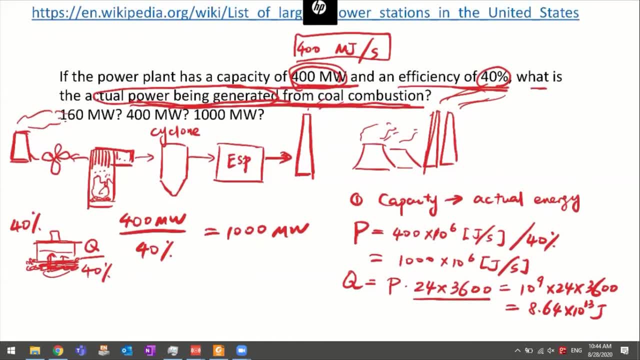 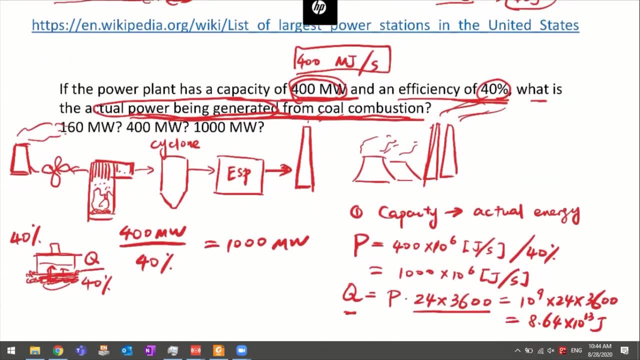 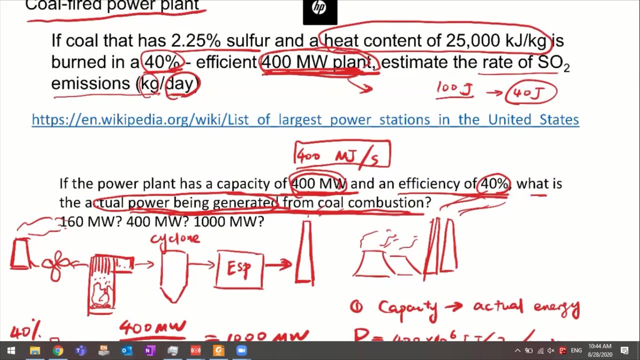 OK, So this is the amount of energy that's coming from the coal combustion during a whole day, Right? So this problem will also give us the heat content of the coal, Right? So basically, it is the energy that can be generated from one kilogram of the coal combustion. 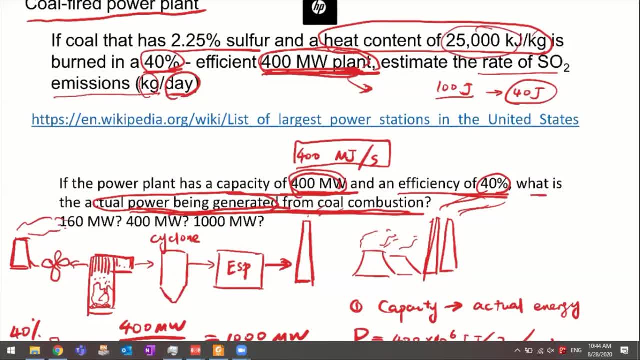 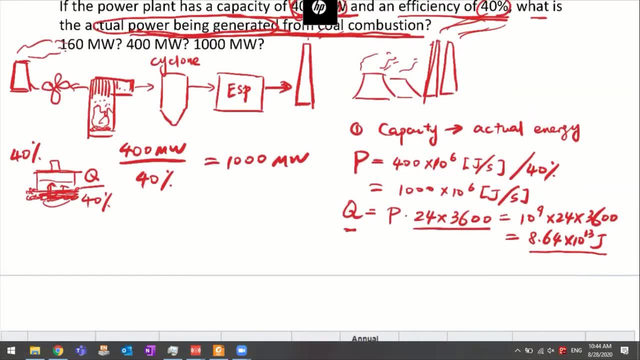 Right, So per kilogram we can generate this amount of energy. It looks pretty large, but if you consider the energy we need for a whole day, right, we can calculate what is the mass of the coal we need for a whole day. 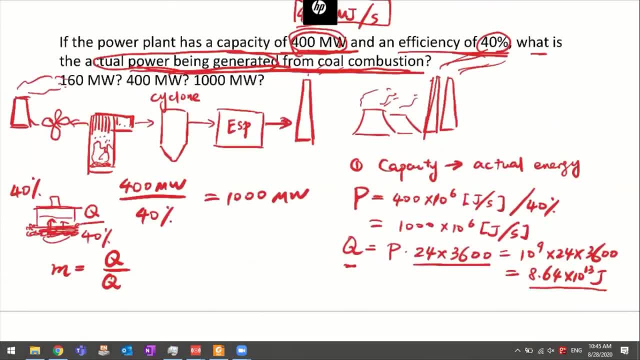 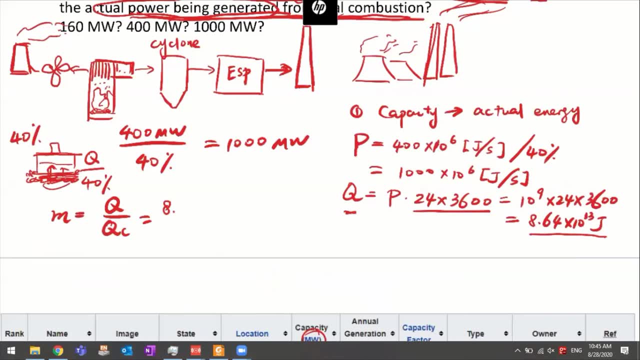 Right. So that's going to be Q divided by this Q. Let's say this is Q, coal Right, QC, OK, So that's going to be 8.64 multiplied by 10 to the 13, divided by 25,000, right. 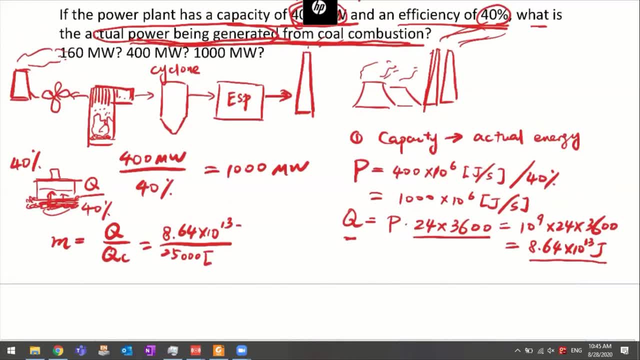 So here, one thing we need to notice is that here we're using joules and here we're using kilojoules per kilogram. So again, we need to make sure that all of these units will conserve right. So if we convert this into kilojoules, then here it should be 10 to the 10th. OK. 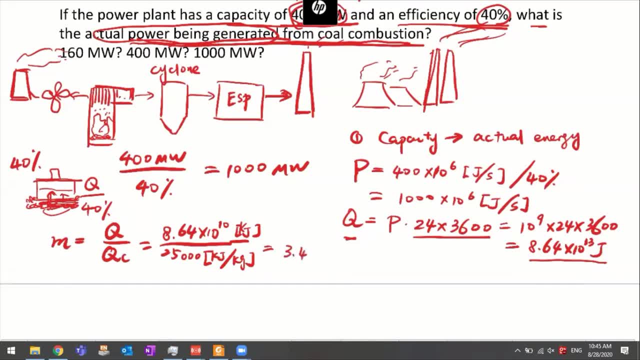 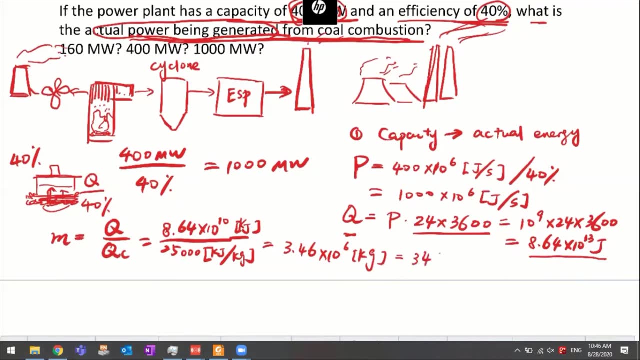 So we can find out that this is actually 3.46 multiplied by 10 to the 6th kilogram. OK, So this is a large amount of mass, right? So it's basically more than 3,000 tons, Right? 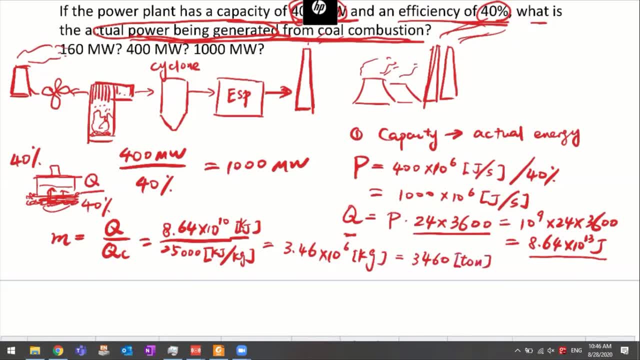 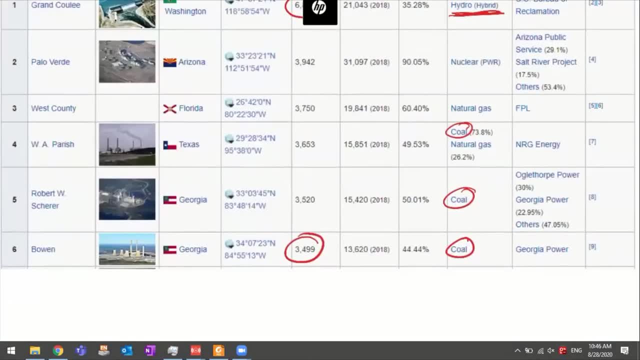 OK, OK. So this is the amount of coal that we have to consume For a whole day. You see, this is this amount of coal that we have to consume even to run this small power plant. Right, If you consider the power plant for this one, then you can imagine what is the amount. 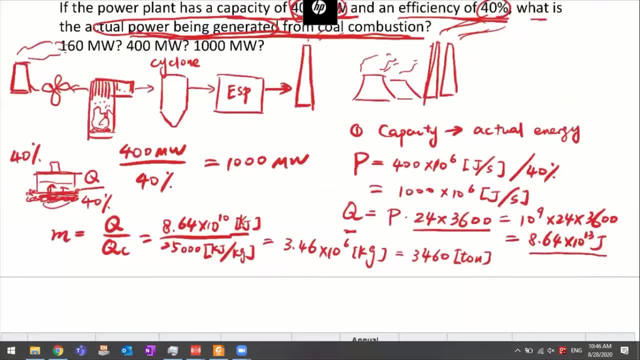 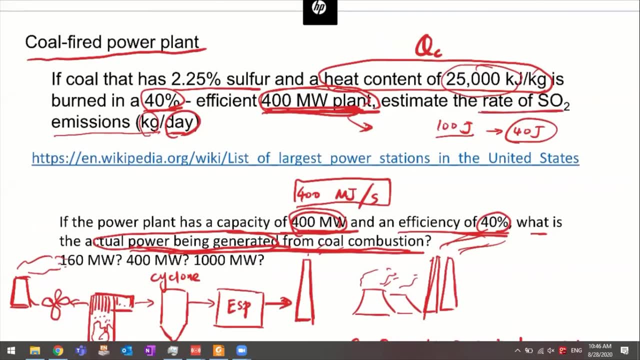 of coal we're burning every day. OK, So here, this is not the end yet. It wants us to calculate what is the emission rate of sulfur dioxide per day. OK, So if we know the mass of the coal being burned per day, 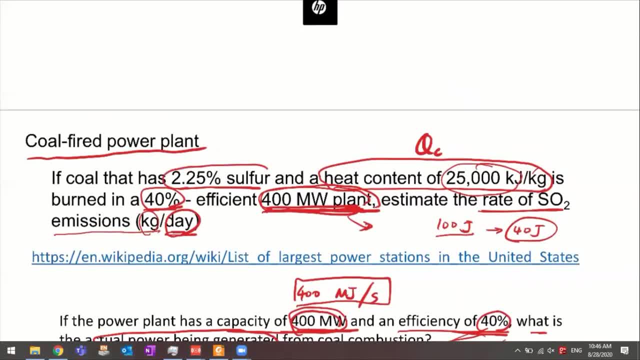 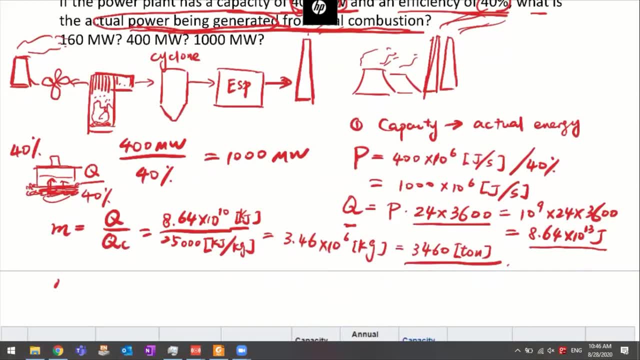 And we also know what is the mass fraction of sulfur in the coal, We can calculate the mass of sulfur that we're generating from these coal right. So that's going to be basically the mass of all of the coal right Multiplied by 2.25%. 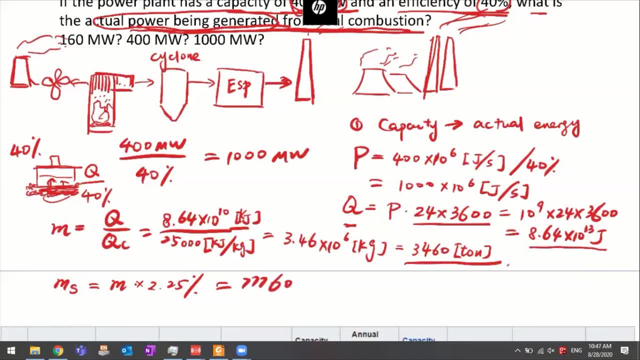 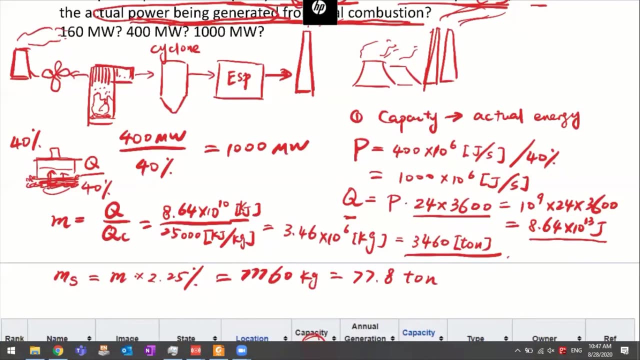 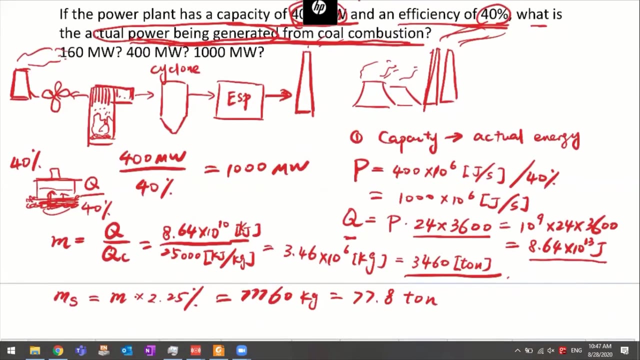 Which is going to be 760 kilogram, Right? OK, So this is more than 77,, let's say 77.8 tons of sulfur every day, right? And finally, it wants us to solve for the sulfur dioxide, Because right now we just calculated the sulfur mass. 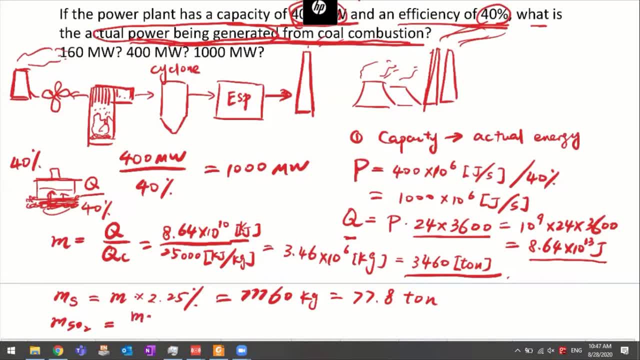 So the sulfur dioxide is going to be the mass of sulfur divided by the molecular weight of sulfur, multiplied by the molecular weight of sulfur dioxide. OK, Which is basically, if we know the sulfur dioxide, that's 64,. right, Sulfur is 32.. 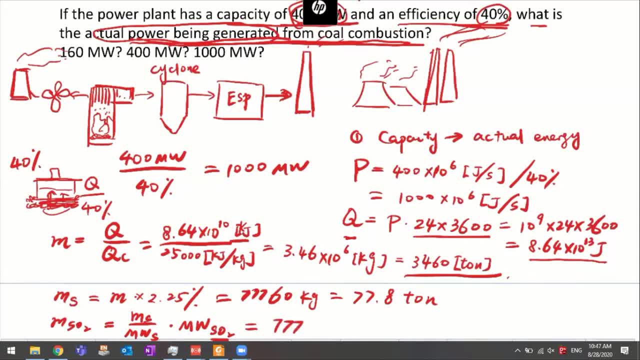 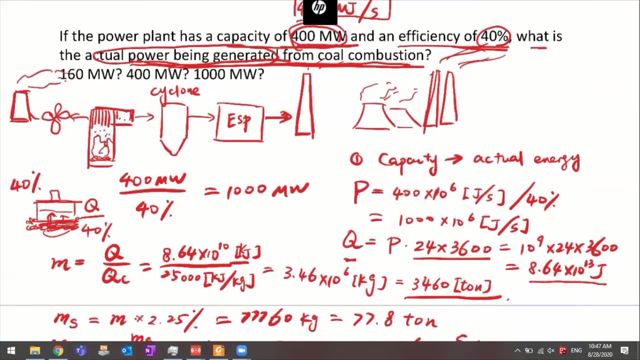 We just need to multiply this value by 2. Right, That's 1.56, multiplied by 10 to the fifth kilogram. OK, If you consider basically what is the amount of sulfur dioxide per day, this is a huge amount.